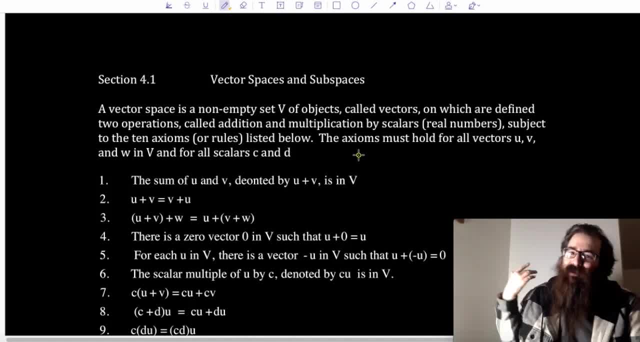 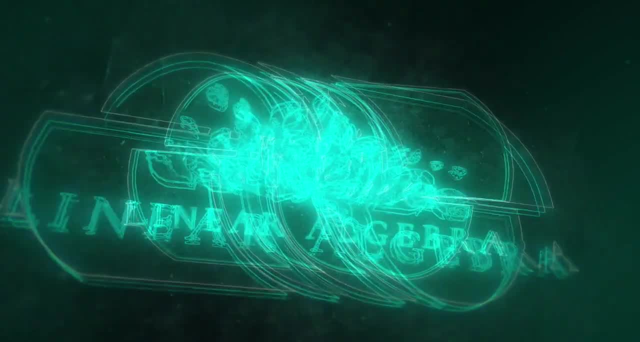 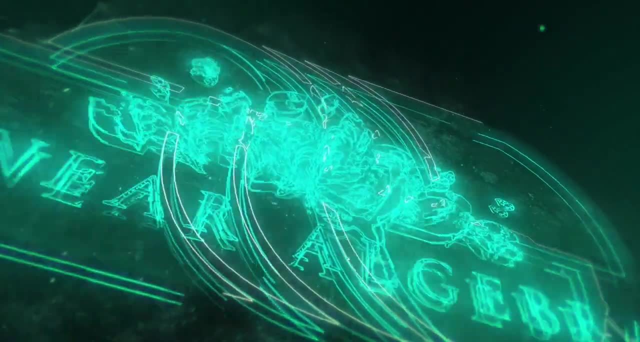 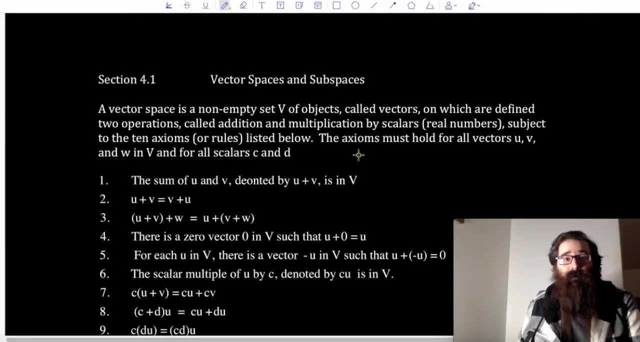 Hey there, LG bros and brouettes. We're doing math on the internet, so don't adjust your TV sets, Let's get mini-er. Welcome. Today we're going to talk about vector spaces and subspaces And we're going to be sort of revisiting some topics, but going a bit further with them and discussing them a bit more in depth. 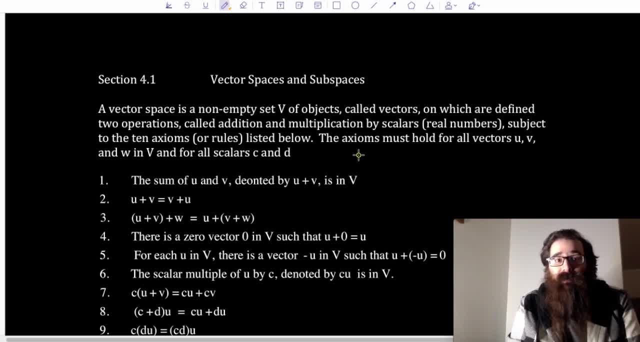 First let's talk about what it means to be a vector space. We've talked a bit about these, but we haven't seen the definition yet. A vector space is a non-empty set capital V of objects called vectors, on which are defined two operations called addition and multiplication by scalars. 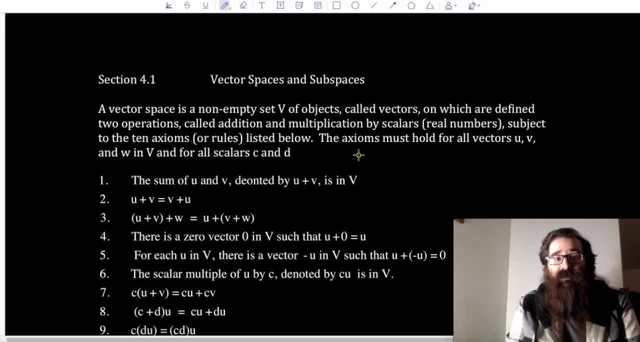 Scalars referring to real numbers, And these are subject to the ten axioms or rules listed. These ten axioms must hold for all vectors u, v and w and for all scalars c and d. So we have vectors u, v and w in the vector space v, and then all scalars referring to real numbers c and d. 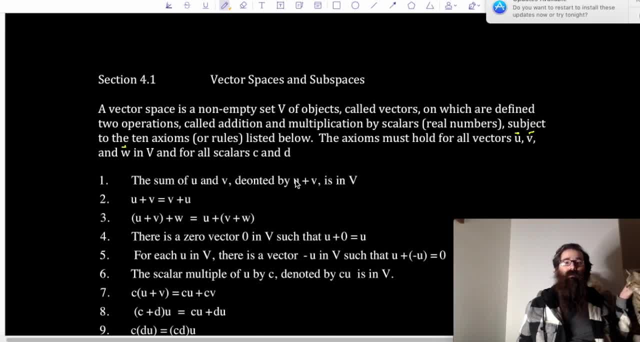 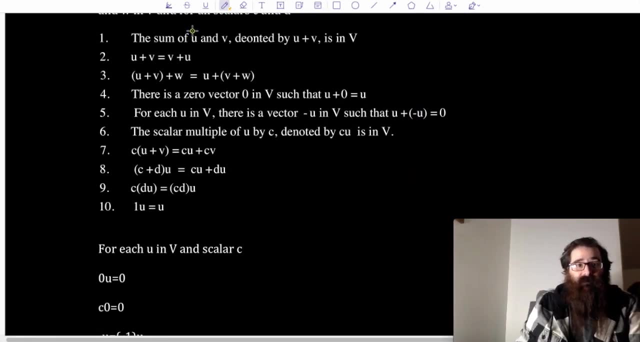 And Lily's here to help us with those ten axioms. Let's talk about it. First of all, we need the sum of vectors u and v, denoted by u plus v is in the vector space, capital V. Second, how, I add, the vectors doesn't matter, right? We have this nice. 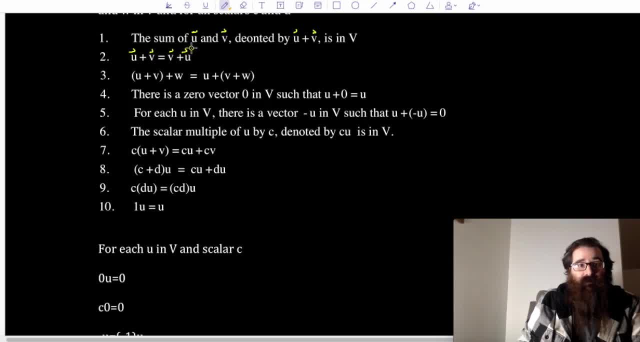 commutative property that u plus v is the same as v plus u. So if I add vector u and then vector v, it's the same as taking vector v and adding vector u to that. We have a nice associativity property there. 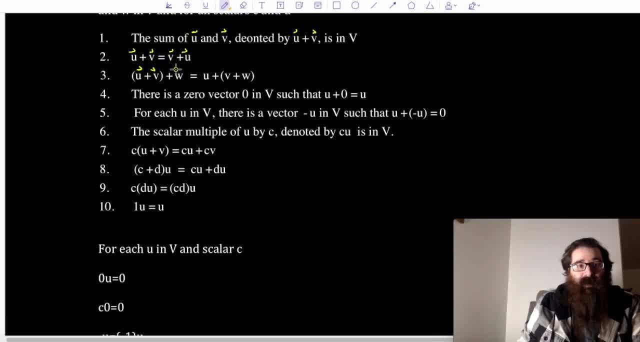 Third: this is if I add vectors u and v together first and then add vector w. that would be the same as adding vectors v and w together first and then adding vector u to that. So a nice associativity property. Fourth, there is a zero vector. 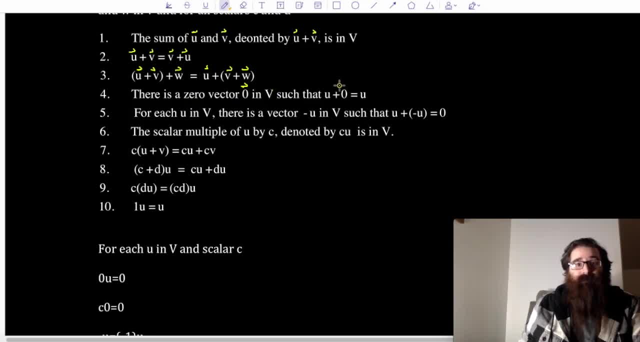 and that's the zero vector in vector space v, such that vector u plus the zero vector is equal to vector u. So we have an additive identity For each vector u. in vector space capital V we have a vector u plus vector u, So we have an additive identity. 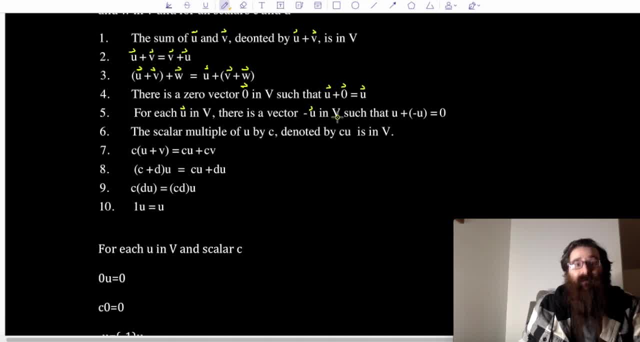 For each vector u in vector space capital V, there is a vector minus u in vector space V, such that u plus minus u gives us the zero vector. So we need an additive inverse: The scalar multiple of vector u by scalar c, denoted by c times vector u is in vector space V. 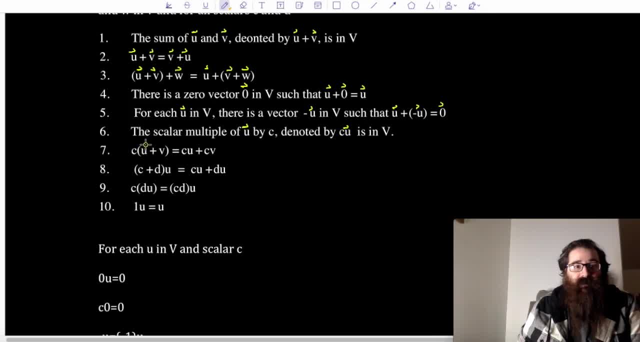 And then now we get some distributive properties, So scalar c multiplied into, and here we have the collection vector u plus v. I have a left distributive line and I have a right distributive line And then I have a right distributive law that says this is the same as c times vector u plus c times vector v. 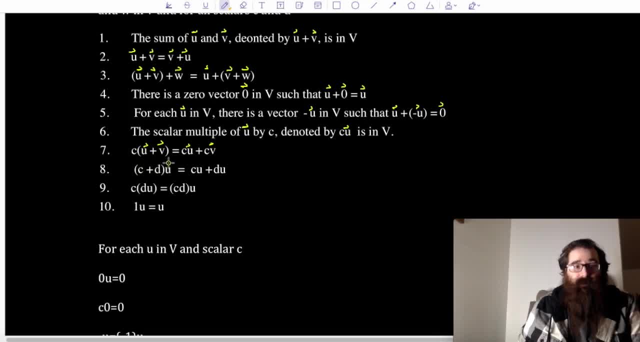 If I have a collection of scalars, so that's c plus d, in parentheses- times vector u, I have a right distributive law That's c times vector u plus d times vector u, And then I can collect scalars a bit differently. 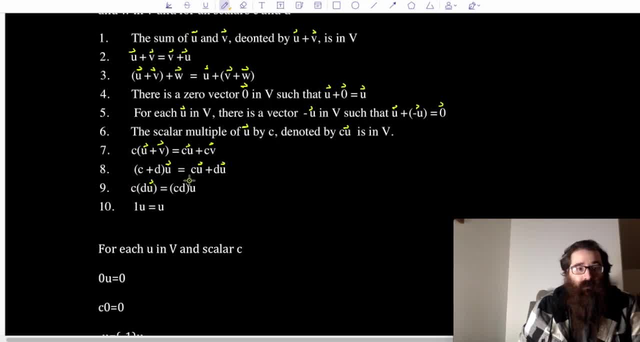 So here we have c times and then the collection d times vector u. I could group c times d and then multiply that as the scalar into vector u. And the last, the tenth property is a multiplicative identity that one times the vector u must give us vector u back. 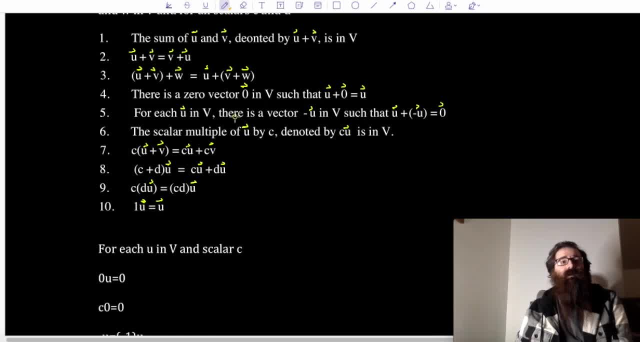 So we get a multiplicative identity. Okay. so, going back over through these properties, you'll notice that a few of them are actually familiar to us And the ones that are, I don't want to say that some of these properties are more important than others. 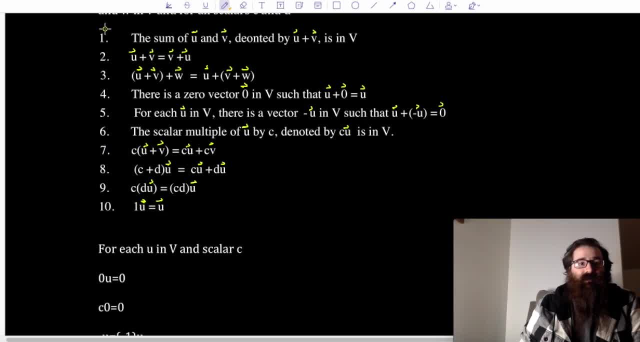 but of this list of ten axioms, the ones that really stick out are one, four and six. That's not to say that we don't need the others, but in fact these three are familiar to us that we need to be closed under addition. 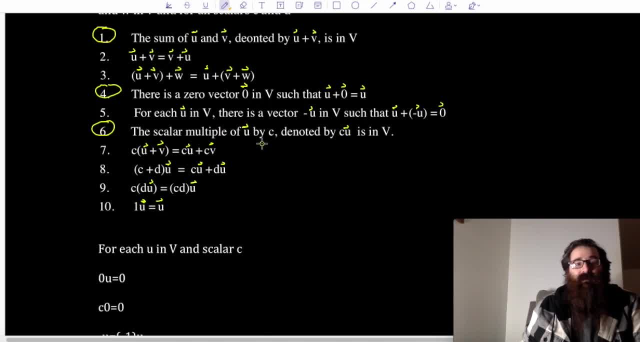 that I need to contain the zero vector and I need to be closed under scalar multiplication. So these are ones that we're familiar with. The rest of these talk about some other properties: right, Commutativity, associativity of adding in the vectors. 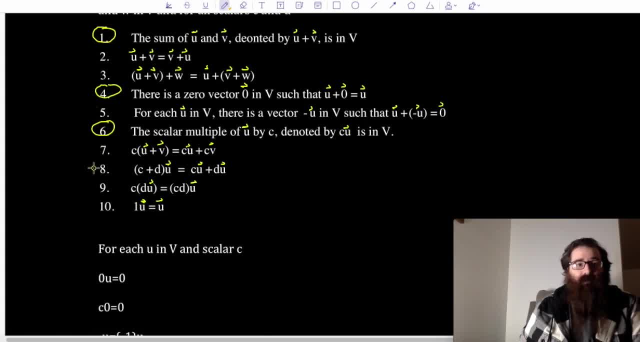 I need this additive inverse. I need a left and a right distributive, I need a distributive law, I need to be able to collect scalars And I need a multiplicative identity. Those you know, those are important as well. 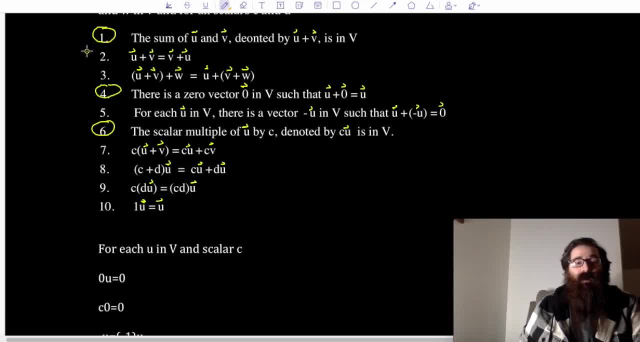 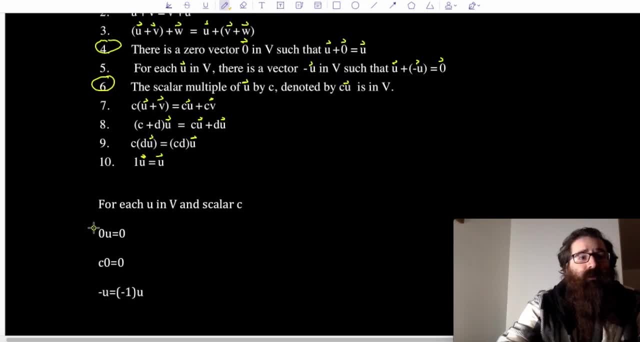 But really, these three properties that we talk about, of these ten vector space axioms, are ones that we've dealt with before, So we're going to actually talk about them a bit more today as well. There are a few other things to clarify here. 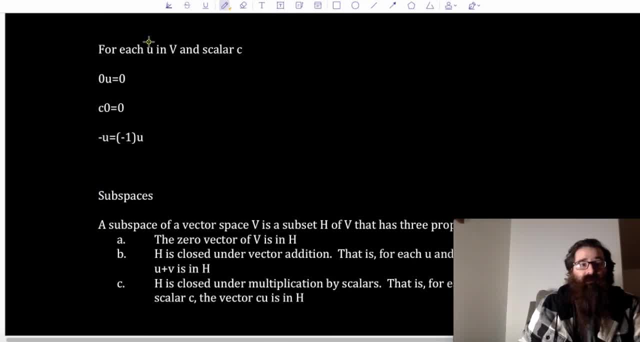 For each vector u in vector space, capital V and scalar c, we need the following: Zero, Zero times vector u is equal to the zero vector. Any scalar c times the zero vector is going to give us the zero vector And when we talk about this vector, negative u. 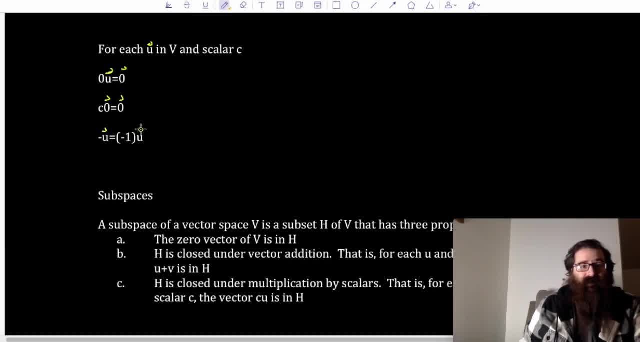 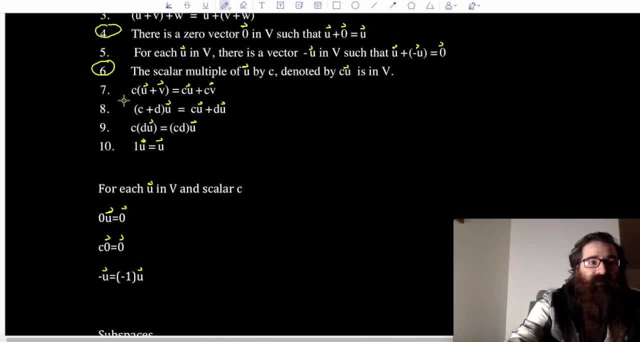 we've talked about that in our additive inverse property, but this is the same as negative one times vector u. So these are three other things you want to consider. But going back to those three vector space axioms- one, four and six- 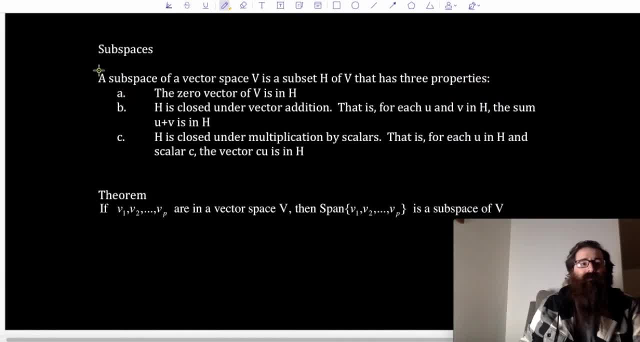 we've seen those before. What do we remember them from? We remember them from subspaces. We would say, well, if I want to show that something is a subspace of a vector space, capital V, this would be a subset H of vector space V that has the following three properties: 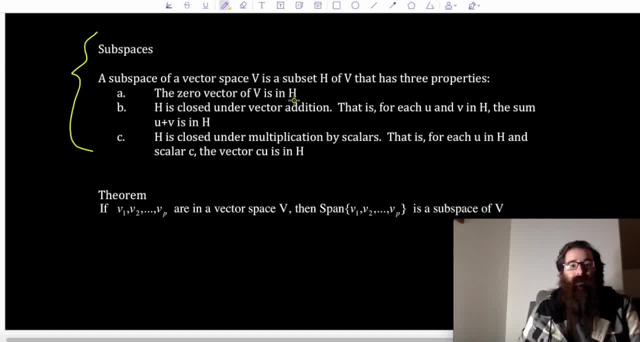 I need that zero vector in that subset H. I need to be closed under vector addition so that means if u and V exist in H, the sum u plus V is in H. And I also need to be closed under multiplication by scalars. 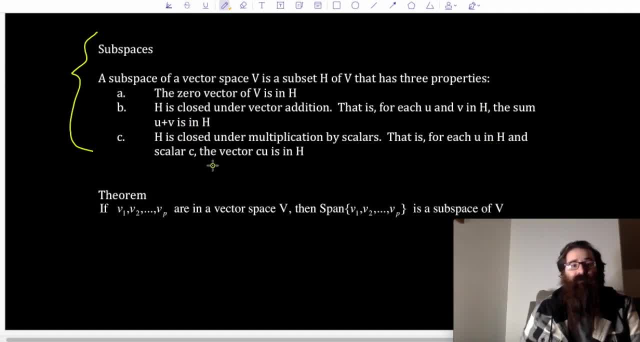 So that means if I have an element u that's in the subset H and any scalar c, any real number c, I need that c times vector u stays in H. We've dealt with this before, so we're really going to be talking a lot about subspaces again. 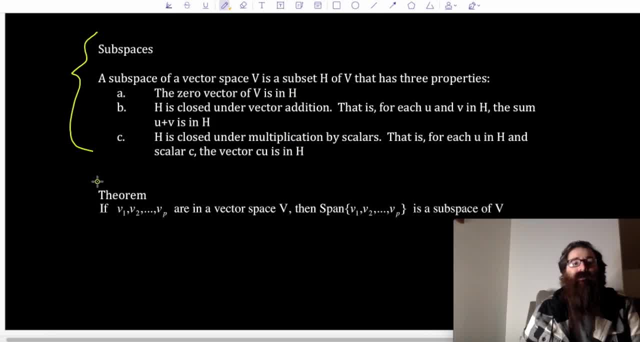 when dealing with vector spaces And we have a very nice theorem that connects these ideas together. It's a very important theorem for the course. We would say, if we have vectors V sub 1, V sub 2, so on and so forth, to V sub p. 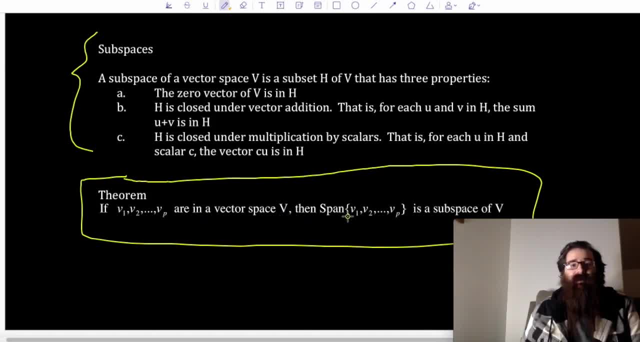 our vectors that live in a vector space, capital V, then the span of those vectors, the span of those vectors is a subspace of vector space V, And that's going to be very important for what we're going to be talking about here today. 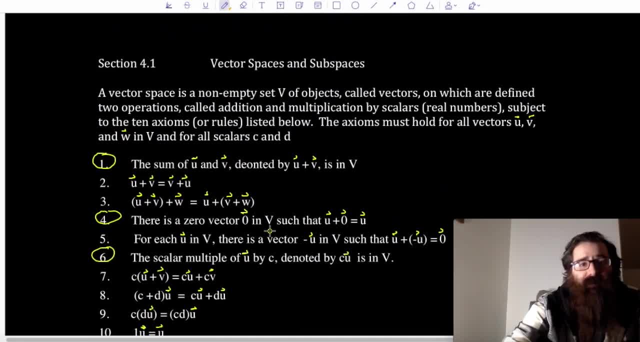 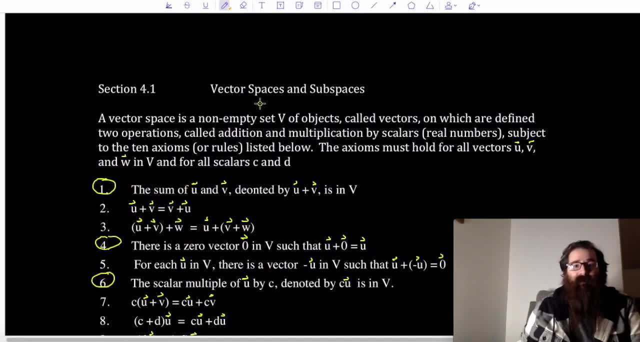 Now, before we start talking about vector spaces in general, let me just give you some ideas of vector spaces that we've already talked about, And some of the best examples of vector spaces are talking about different spaces dealing with real numbers, So an example of a vector space could just be: 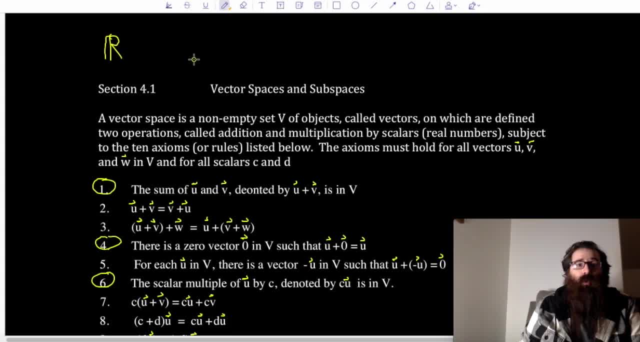 R, our real number line. Or if I want to talk about our Cartesian plane, R2, it's another example of a vector space. If I want to work in three dimensions, R3 is a vector space, and so on and so forth. 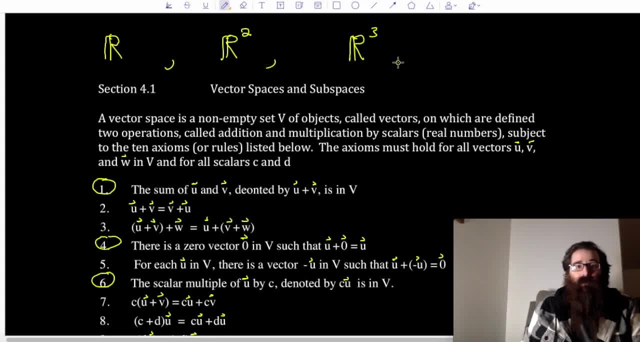 It doesn't have to stop here. R, R squared, R2, R3,, for example, are all vector spaces, But I can continue on And really, when we talk about vectors and the size of those vectors, we can talk about the vector space that they belong to. 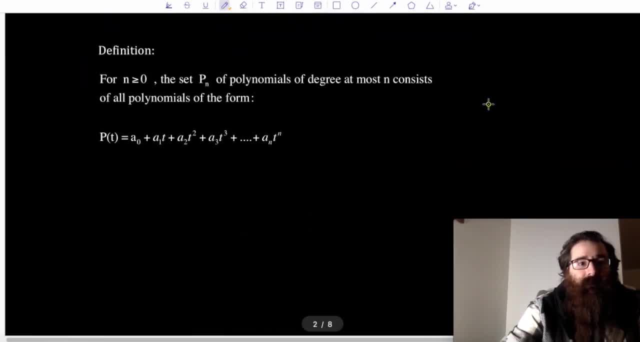 is really the idea, But that's not the only possibility. We can also talk about a polynomial space as a vector space. So here we have a definition of this. For n greater than or equal to 0,, the set P sub n. 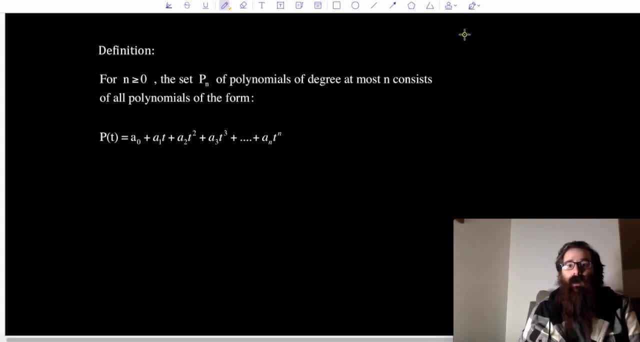 so this would be sort of bold. it's very similar to vector space Rn. In general we say vector space Rn, where we have R and then we have a superscript n. polynomial spaces: we use P instead of R. 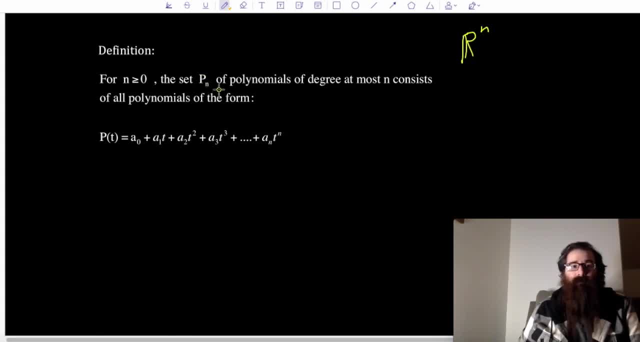 and then we have a subscript n. But the set Pn of polynomials of degree, at most n, consists of all polynomials of the form: polynomial P at t equals a sub 0 plus a sub 1 times t plus a sub 2 times t squared. 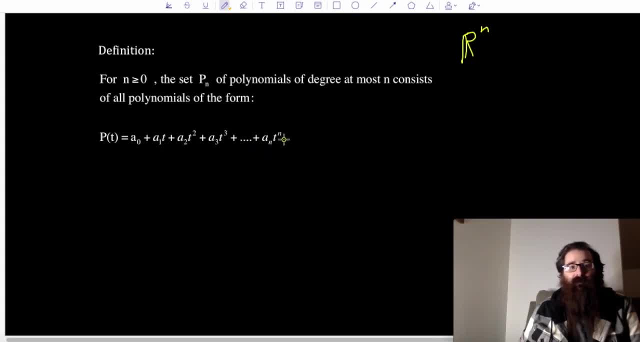 plus a sub 3 times t, cubed plus so on and so forth, plus a sub n times t to the power of n. So here we're talking about polynomials of degree at most n, And there's something important to sort of mention here. 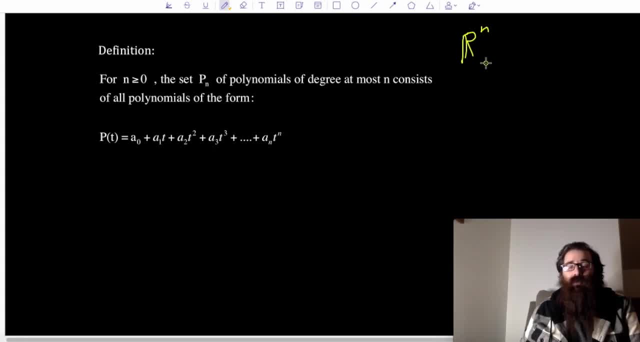 about how polynomial spaces relate to sort of more traditional vector spaces like Rn for example. But before talking about that let's just sort of go through some ideas here. So I'm not going to go through all ten axioms to show that a polynomial space 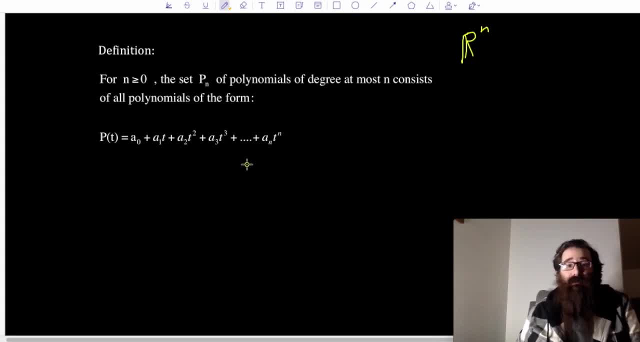 is in fact a vector space. You could certainly do that, but let's take a look at at least those three important properties that we're sort of showcasing that we've already dealt with with subspaces. So if I go ahead and pick on, 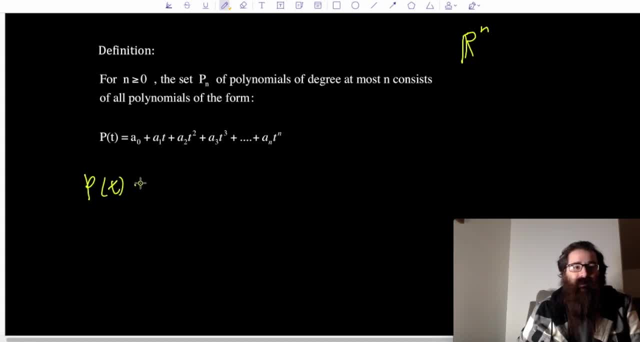 let's say a polynomial P at t, which here I'm going to go ahead and say: well, this is just. we have real numbers, a sub 0, a sub 1, a sub 2, so on and so forth. 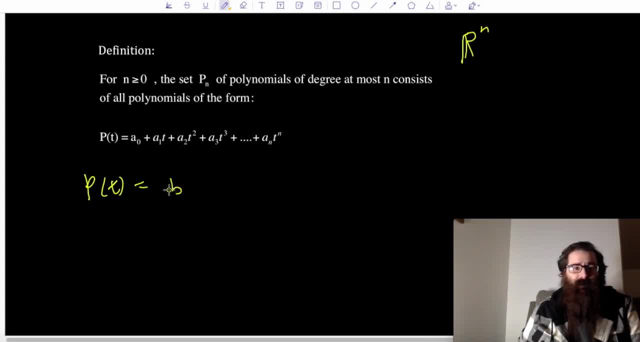 to a sub n. I mean in this case, let me just call it. for example, I'll do b sub 0, b sub 1t, b sub 2t squared, b sub 3t cubed, plus so on and so forth. 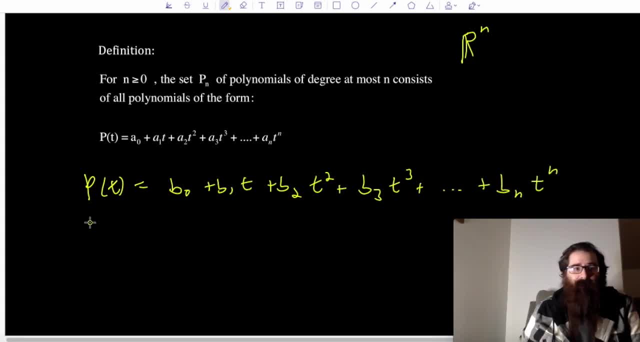 So we get to the end: b sub n, t to the power of n. And if I take another polynomial, q at t and say this is of the same form: so some constant c sub 0 plus c sub 1 times t. 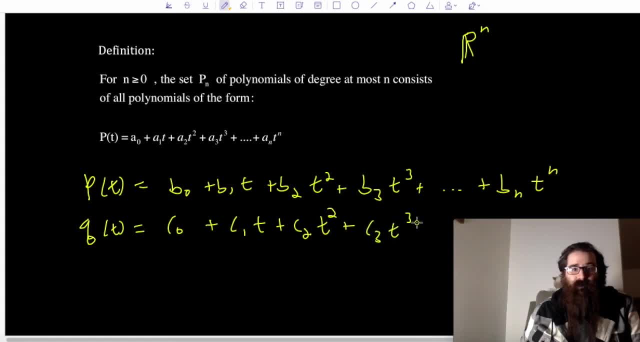 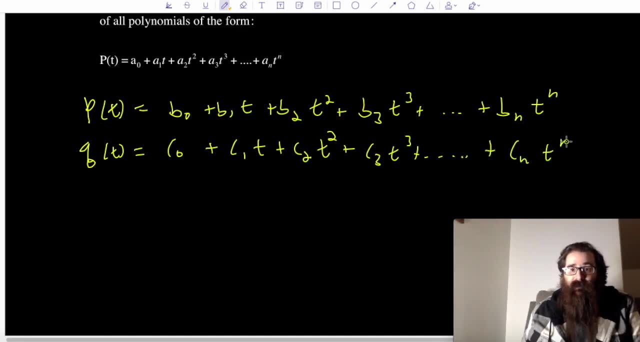 plus c sub 2 times t squared, plus c sub 3 times t cubed, plus so on and so forth. plus c sub n times t to the power of n. These are both examples of polynomials that meet this description, where you know all the b values. 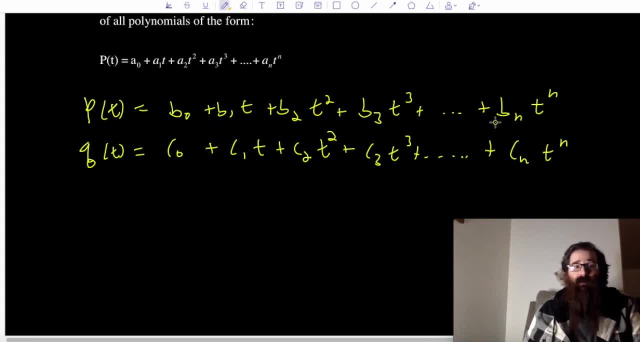 and all the c values are just real numbers. These are both polynomials of degree, at most n. If I were to add these together. so what if I were to take these two elements that exist in the polynomial space and add them together? what is that going to give me? 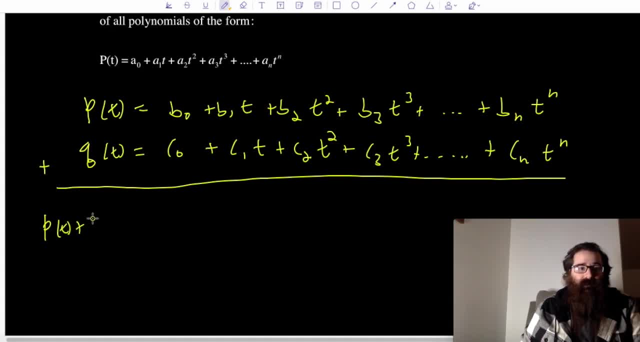 Well, that's going to give me some new polynomial, namely p at t plus q at t. What's going to happen here is I'm going to add and sort of collect like terms, and I'll skip over some of the steps there. 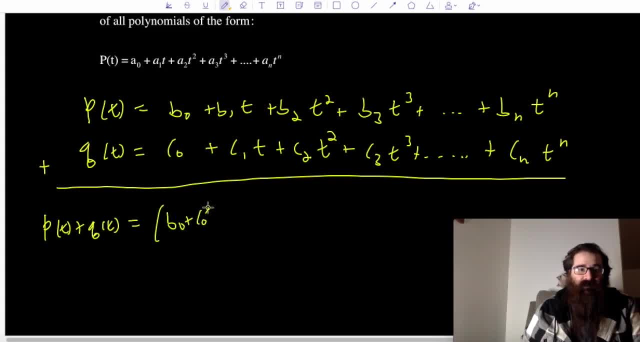 but I'm going to have this constant term: b sub 0 plus c sub 0, and I'm going to have a coefficient on t. when I add these together, That's going to be b sub 1 plus c sub 1 times t. 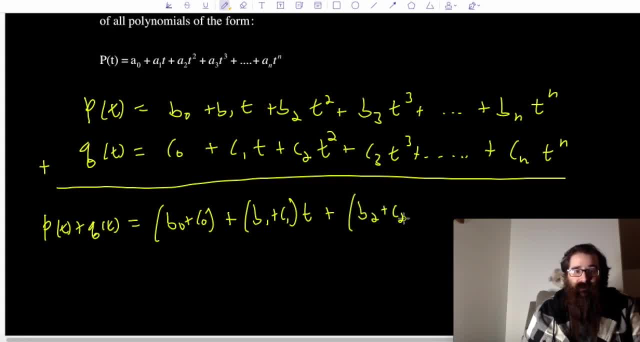 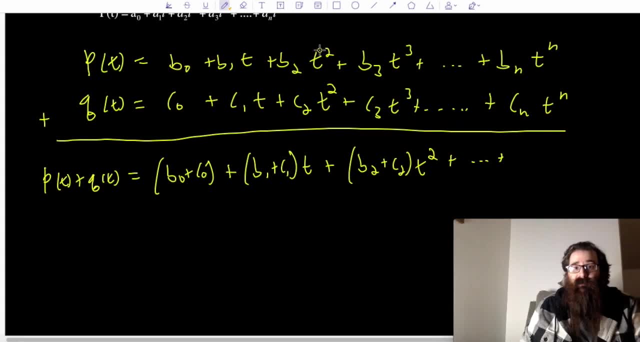 I'm going to have a coefficient on t squared, b sub 2 plus c sub 2 times t squared. and just so I don't run out of room, I'll do plus dot, dot, dot, and then you know. same thing with adding the t cubed terms. 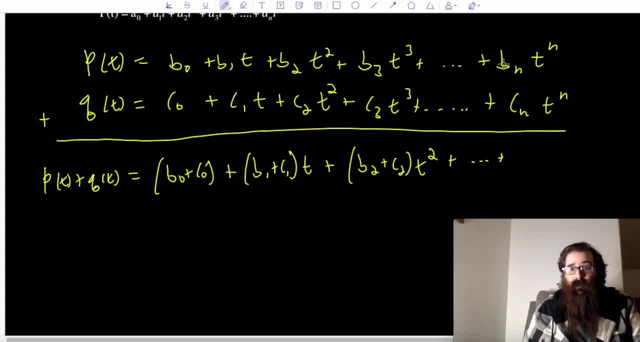 I can collect the coefficient b sub 3 plus c sub 3, and then at the end here my coefficient on t to the power of n. that's going to be b sub n plus c sub n, and then quantity times t to the power of n. 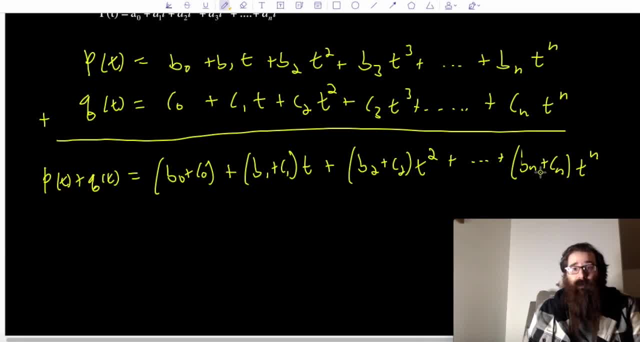 And adding these real numbers together for my coefficients and my constant term. just give me some other real numbers. We could, you know, rename it if I'd like to. I could say: well, this is some constant, a sub 0, plus some constant- a sub 1 times t. 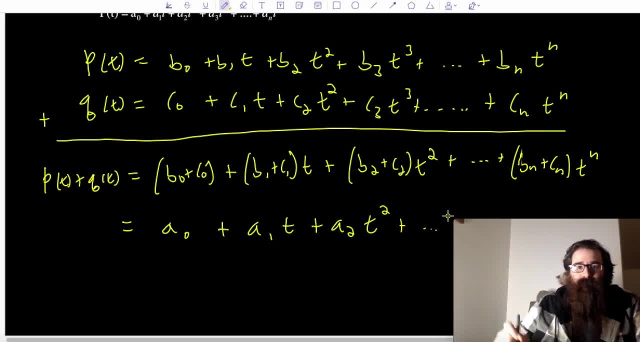 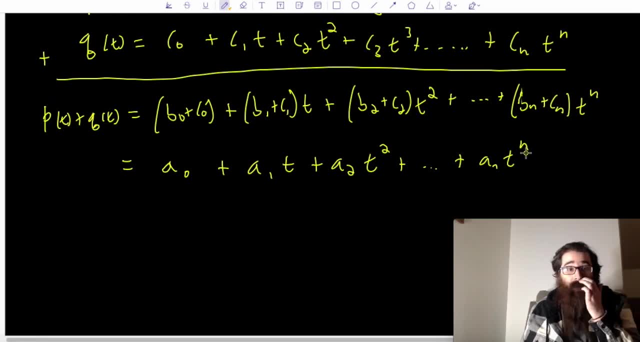 plus some constant, a sub 2 times t squared plus so on and so forth, plus some constant, a sub n times t to the power of n. So adding two polynomials together in this polynomial space gives me another polynomial of the same form. So I stay inside of the space. 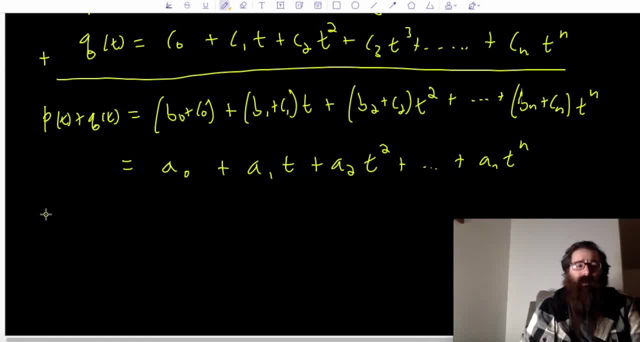 So that first property is there. What if I want to talk about the zero element? Well, in this case the zero element is really just the zero polynomial, And I can have that zero element in my polynomial space. It's going to be very boring. 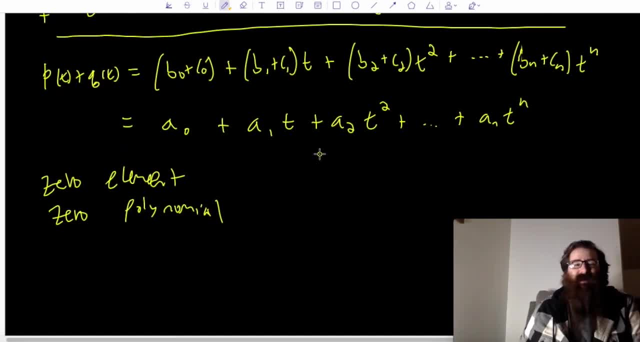 Now, keep in mind t is going to be our variable and I don't want to say anything or impose any restrictions on t. t can be whatever it wants, to be right. We think of a polynomial, We're not thinking of a constant. 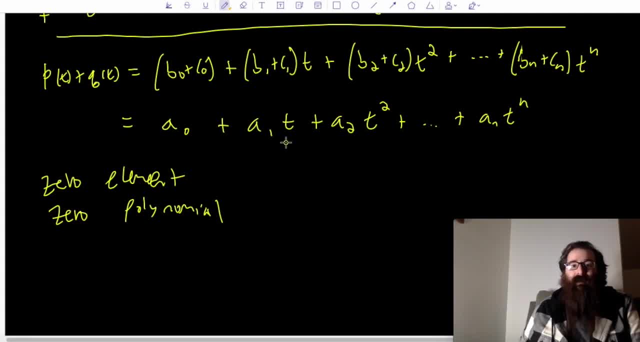 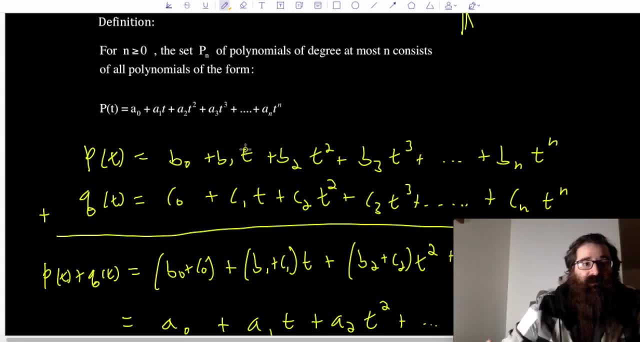 We're not thinking of a specific value for the input of it. We're saying we're just doing the polynomial in general. What I do have control over, though, are the coefficients, the scalars right, And I do have a zero element in my polynomial space. 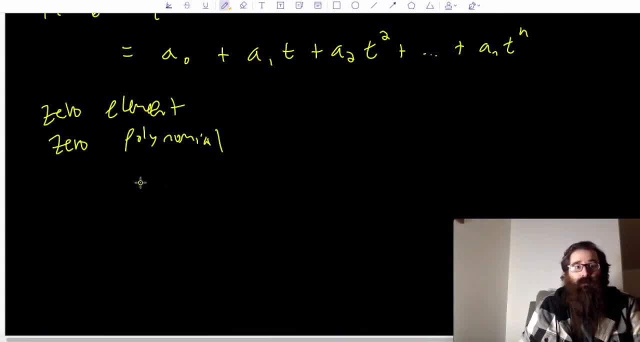 which would namely be the zero polynomial 0 plus 0t, plus 0t squared, plus 0t cubed, plus so on and so forth, plus 0 times t to the n, And it is sort of underwhelming. but certainly if a sub 0, a sub 1, a sub 2,. 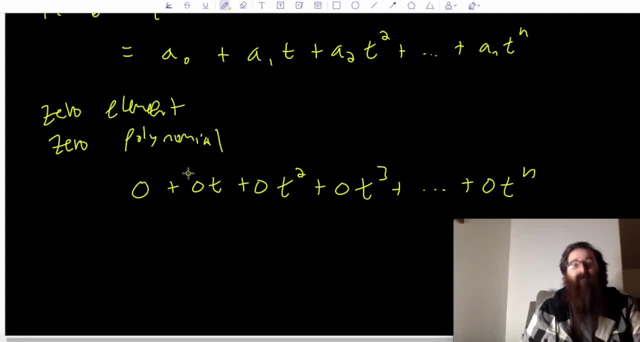 so on and so forth, to a sub n are all zero, then that gives me the zero polynomial, which is the zero element in my polynomial space. And then we can talk about one more of these properties. Remember, there's 10 of them in total. 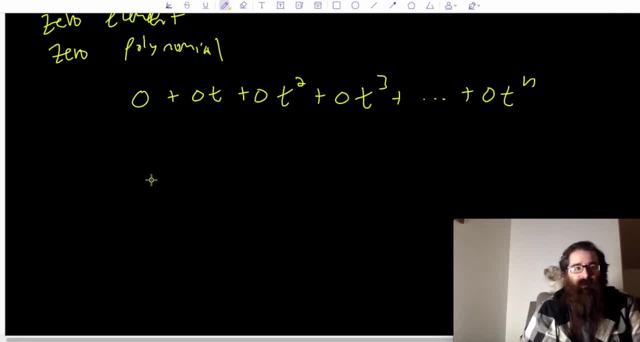 but we're just going to focus on the three big ones for now, Because I'm going to run out of space soon anyways. But what about being closed under scalar multiplication? Well, if I take a polynomial p at t, let me just call this, you know. 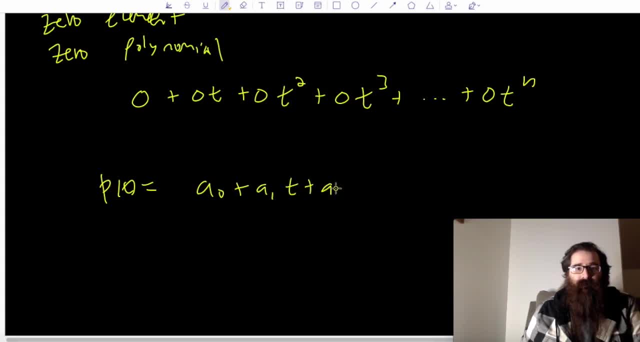 a sub 0 plus a sub 1t plus a sub 2t, squared plus, so on and so forth, plus a sub n times t to the n, so a polynomial of degree at most n, and I multiply this by some scalar c. 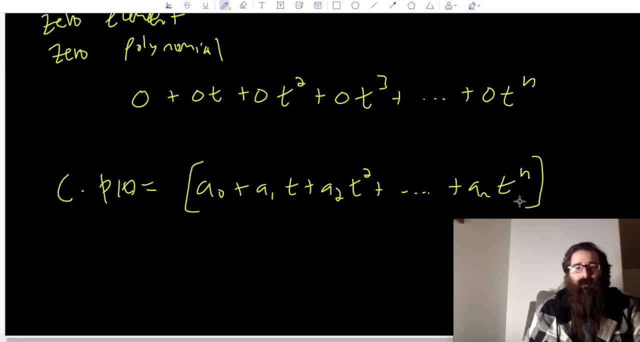 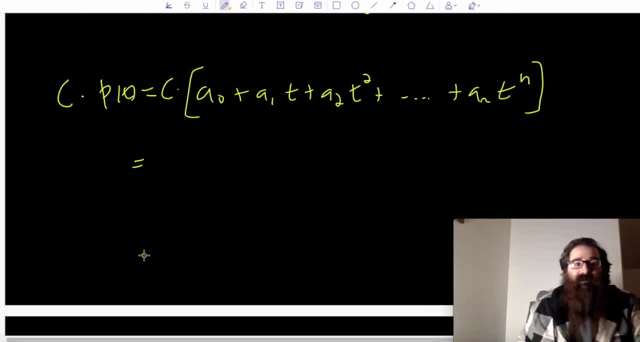 I'm going to say, well, I can do that, I can multiply by a scalar c, and then I can think about distributing this through. And how is that going to look when I distribute c through? Well, I'm going to get c times a sub 0. 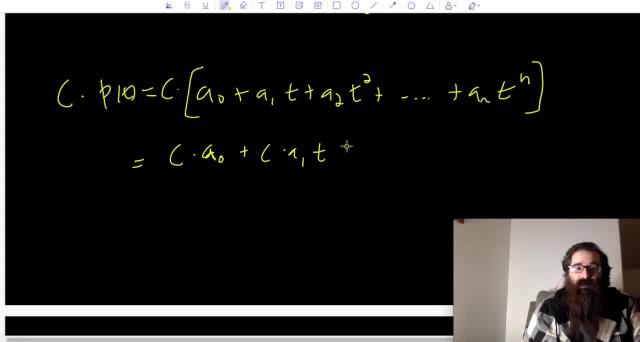 plus c times a sub 1t, plus c times a sub 2t, squared plus so on and so forth. plus c times a sub n t to the power of n, And all of these values where I'm taking a real number, some a, a 0, a 1,. 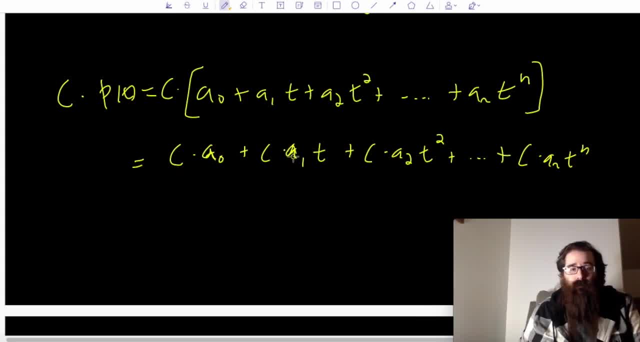 so on and so forth, and multiplying it by another real number, it's going to give me a real number. So I can go ahead and, you know, give this a new nickname. I could use sort of party hats for my notation. 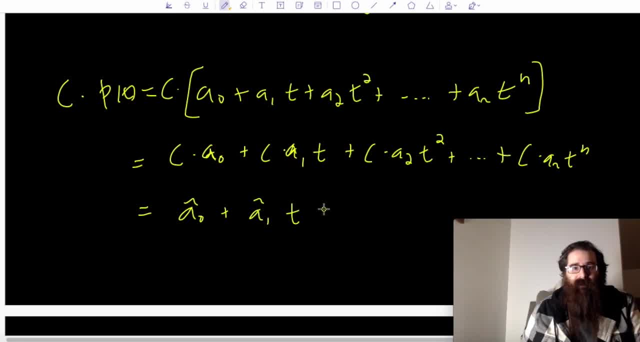 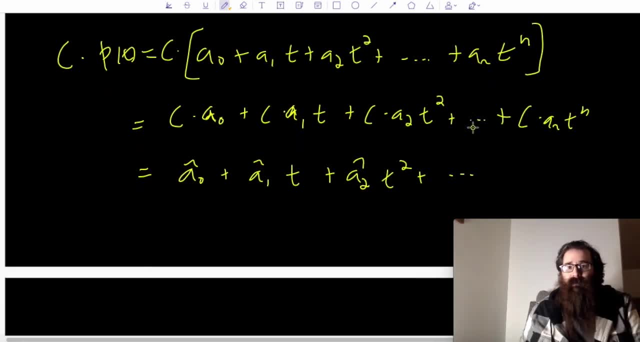 I could say: well, a sub 0 hat plus a sub 1 hat times t, plus a sub 2 hat times t, squared plus so on and so forth, plus a sub n hat times t to the n, where these are all real numbers. 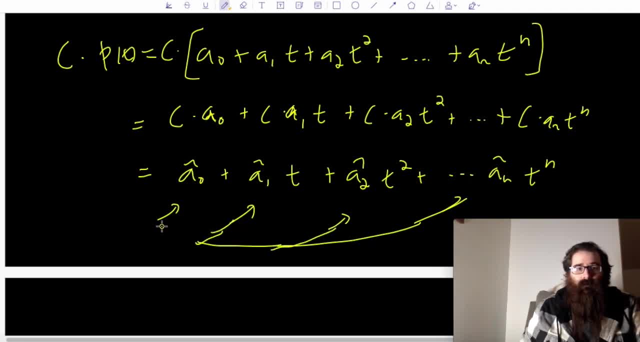 These are still all real numbers, So I stay in that polynomial space And you could show that those remaining seven axioms hold true as well. but the idea really is that I can show that this is a vector space, So I can work with a polynomial space as well. 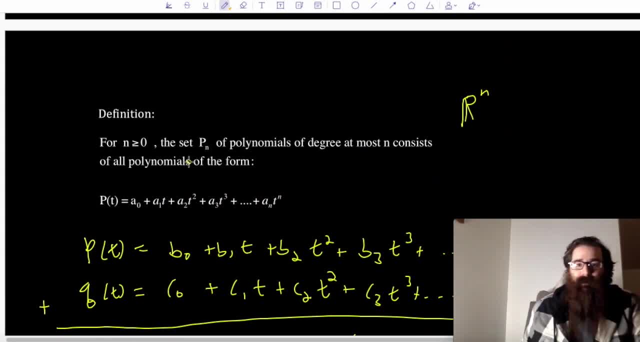 What's very interesting about the polynomial space is that we could make the following claim: We could say that polynomial space p p with this subscript n is going to be isomorphic to traditional vector space r n plus 1.. You'll think: well, why is that? 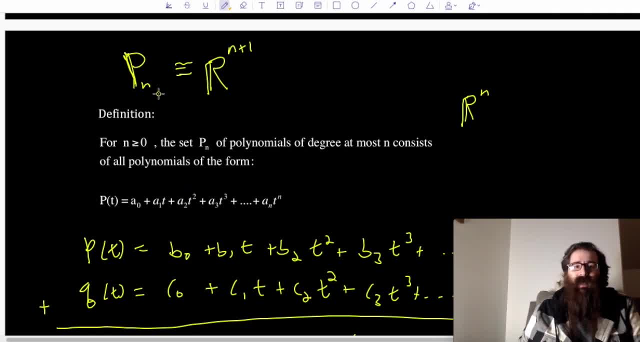 Well, when I already tell you a polynomial of degree, at most n, you already have a very basic understanding as to how this looks. In fact, you know most about it. The only things that you don't know are: what are the coefficients? 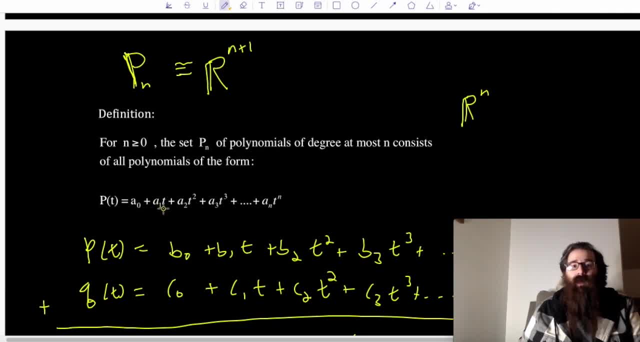 and what does the constant term look like? So if I really want to strip away the unnecessary information about a polynomial of degree at most n, then what I can do is I can just describe how those constants and coefficients look, So we could assign this polynomial. 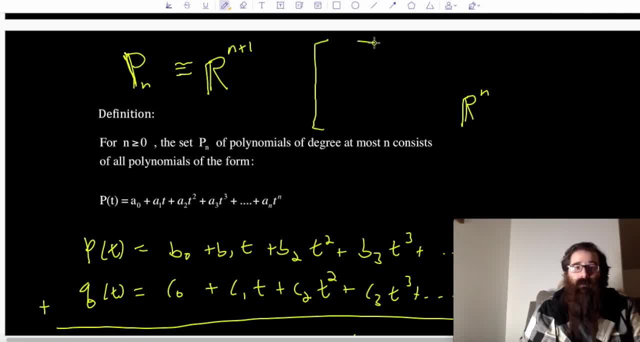 to a vector. How would that vector look? Well, I need to know the constant term: a sub 0.. I need to know the coefficient on t- a sub 1.. I need to know the coefficient on t squared: a sub 2, so on and so forth. 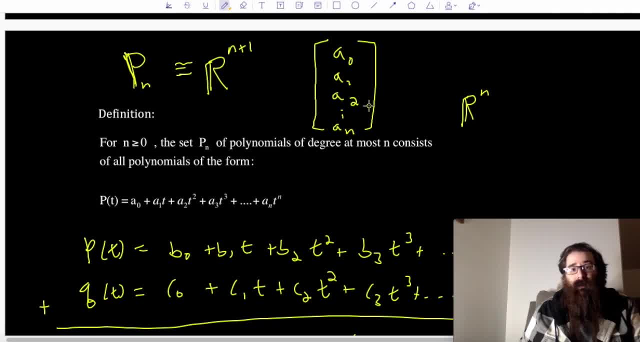 And then I need to know the coefficient on t to the n, a sub n. So all I need to know are these constants and coefficients. I need to know, well, what are those. And if I know what those are, then I can build the polynomial myself. 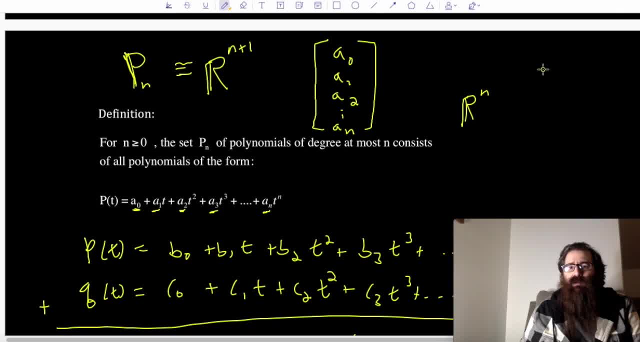 And you think: well, if I tell you I have some quadratic, some polynomial of degree 2, what do I need to know? All I need to know is the constant and the coefficients. So let's say I have a function, right? 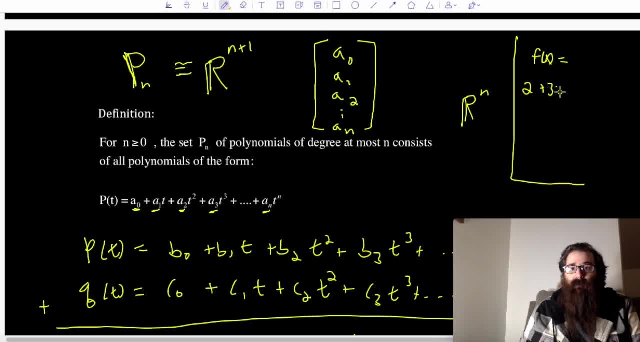 A quadratic. Let's say I have something like 2 plus 3x plus 4x squared. I don't really need you to tell me the form of it if you're saying that it's a polynomial of degree 2.. The only things that I need to know. 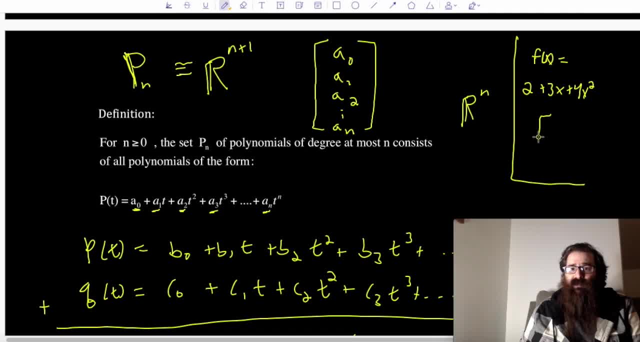 are what those constants and coefficients look like. So we're saying that we can actually just assemble the information into a vector, for example 2, 3,, 4, and I'll know the order it should go in. It should be 2 times x to the 0,. 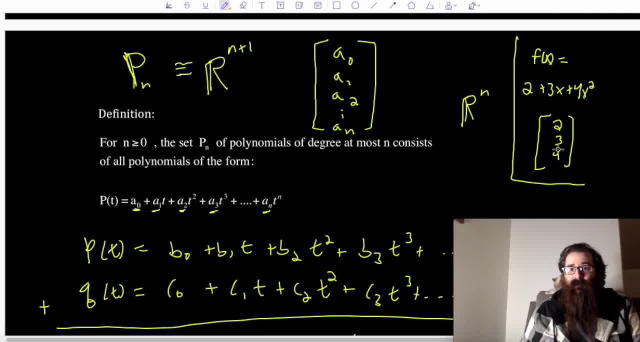 my constant term, plus a 3 times x to the 1st and a 4 times x squared, And that's kind of the idea. But we'll notice that in general, if I'm talking about a polynomial of degree, at most n. 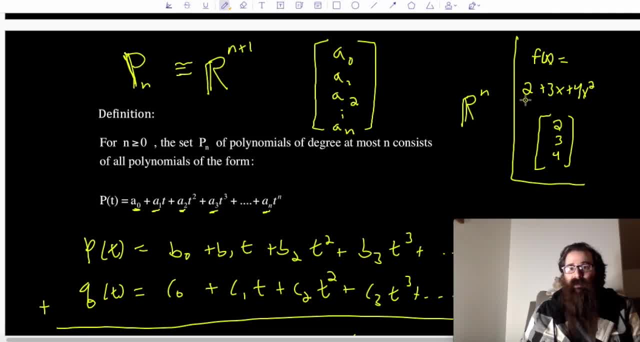 there really needs to be n plus 1 terms here, Like, for example, if I have a polynomial of degree 2, I need 3 terms to designate because I have this constant term to worry about as well: The x to the 1st term and the x squared term. 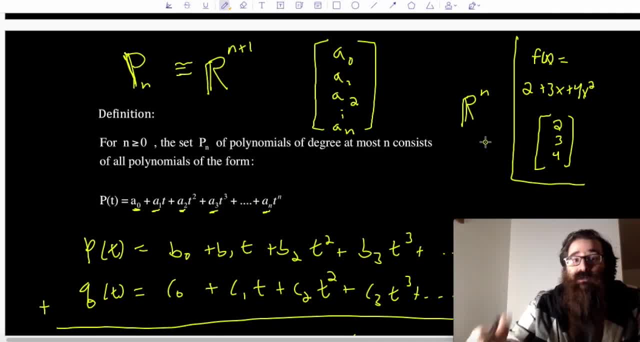 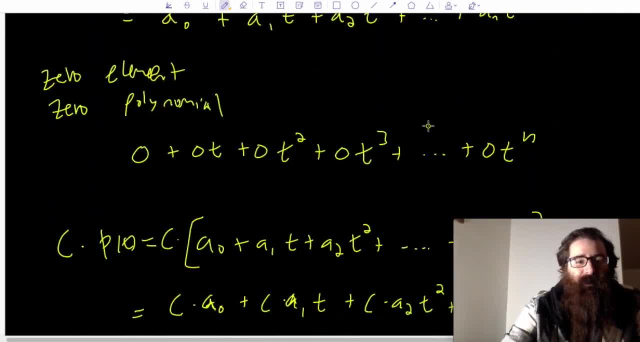 I need to know what those constants and coefficients look like. So we have a really nice way of thinking about a polynomial space in terms of a traditional vector space anyways. So you might think, well, this isn't really much different and you're not really wrong. 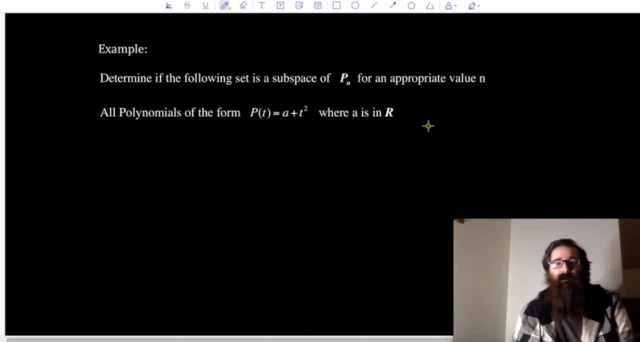 Let's work with these polynomial spaces a bit, talk a bit about them further. So I want to determine if the following set is a subspace of Pn polynomial space with degree at most n for an appropriate value of n, And I want to talk about all polynomials. 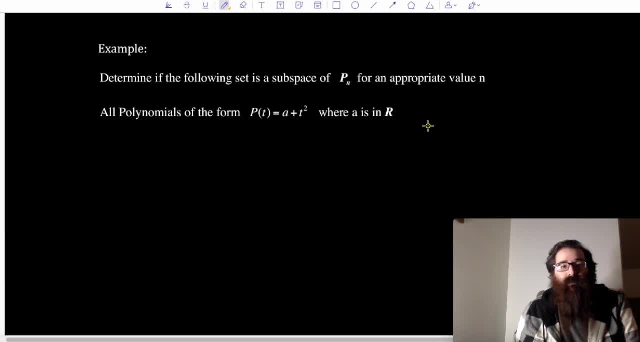 of the form p at t is equal to a plus t squared, where a is just some real number, a is an r, And so now, since I have a plus t squared, I notice the degree of this is at most 2.. 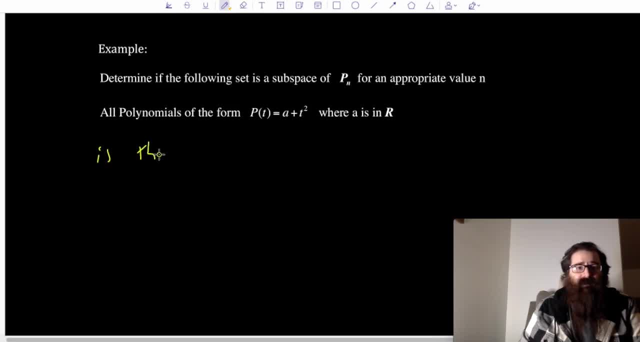 So I want to know: is this a subspace of polynomial space? P2?? So that degree at most 2.. Now, in order for this to be a subspace of a polynomial space, I need those three axioms to hold true. 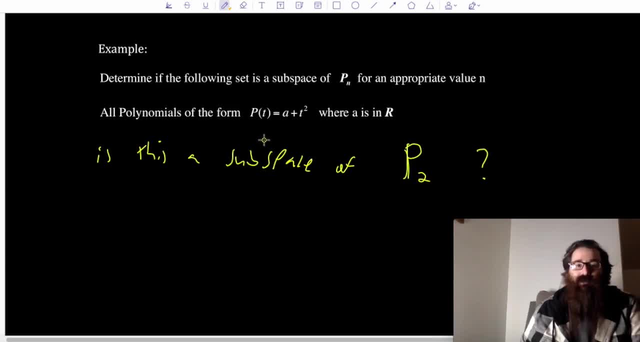 I need those three pieces right. I need to make sure I'm closed under addition. I need to make sure I have the zero element. I need to make sure that I'm closed under scalar multiplication. Now, in this example, depending on where I start with this, 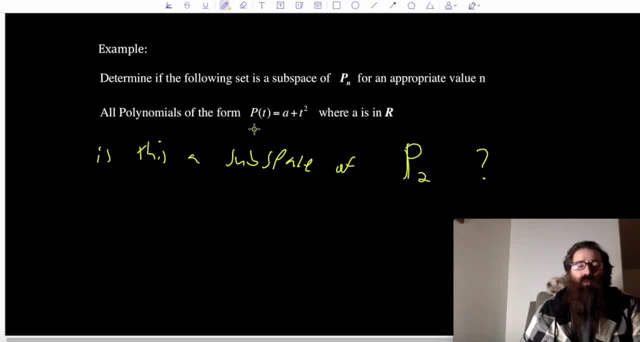 I don't think it's going to work out so nicely. So, for example, if I work with addition, first, let's say I take some example of a polynomial, let's say some number, b plus t squared, and then another polynomial, call it q at t. 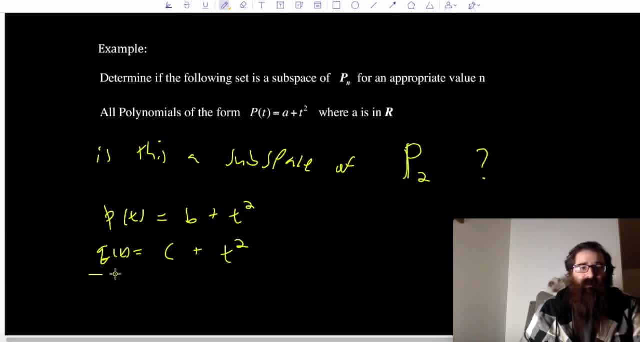 let's say some constant c plus t, squared. If I add these together, I want to know: am I going to stay in the polynomial space? Am I going to stay in? well, really, am I going to stay in my alleged subspace? 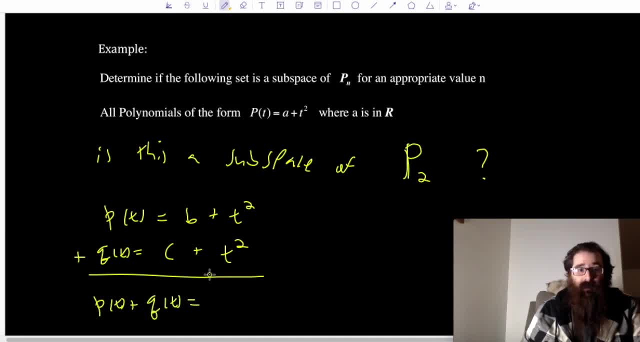 my proposed subspace. I don't know if it is one or not. Let's say: well, I add the constants b plus c gives me some constant term, and then adding t squared and t squared gives me two t squared, And this is a bit of a problem. 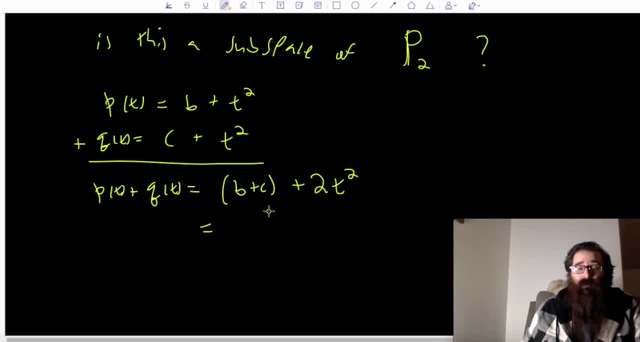 We'll see why it's a problem. When I add a real number to another real number, it just gives me some other real number. so I can call this a plus two t squared. But the issue is actually this: coefficient on t squared. 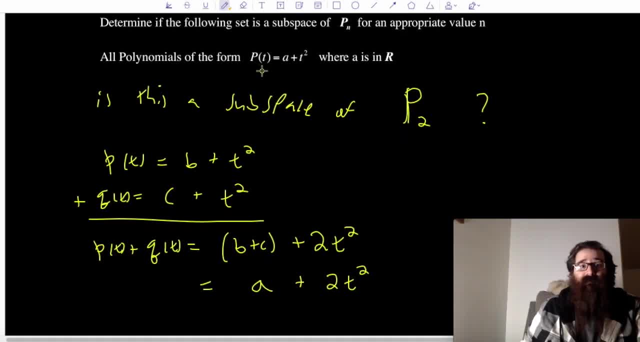 In order for me to stay in the description that I'm given, we're saying all polynomials of the form. the polynomial has to be a constant plus t squared. It has to look like that. It has to be a number plus t squared. 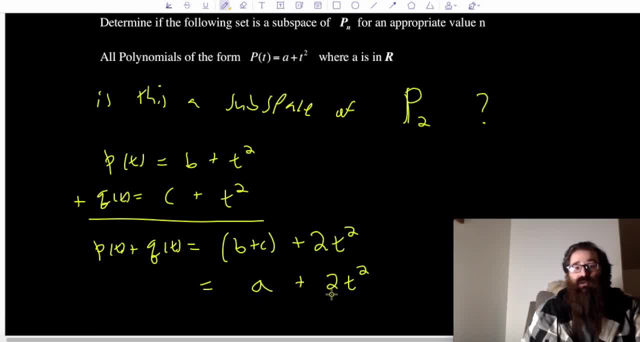 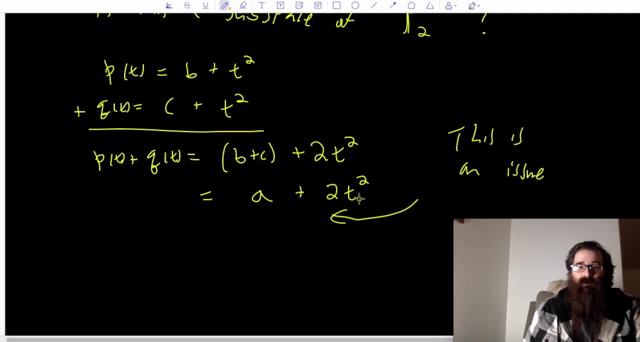 I'm not allowed to have a number plus two t squared. No one mentioned anything about a two in front of the t squared. That's not allowed, So this is an issue, So we'll save this. This is an issue, So this actually fails at this point. 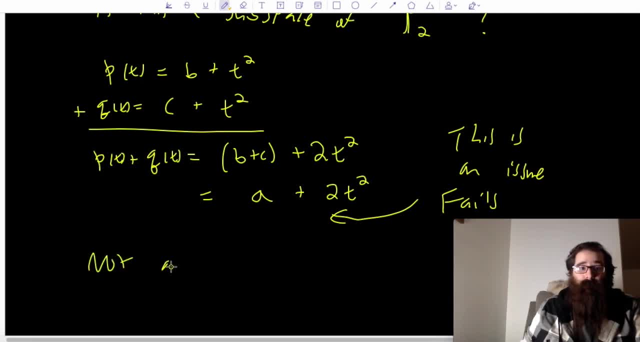 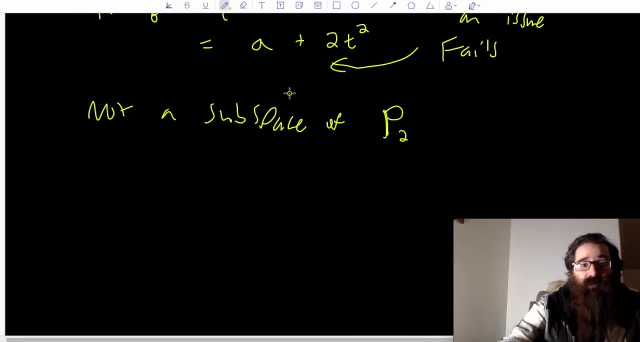 So this is in fact not a subspace. It's a polynomial of polynomial space p2.. What's interesting is that you would notice that all three of the properties fail If I take a polynomial like this and try to multiply by a scalar. 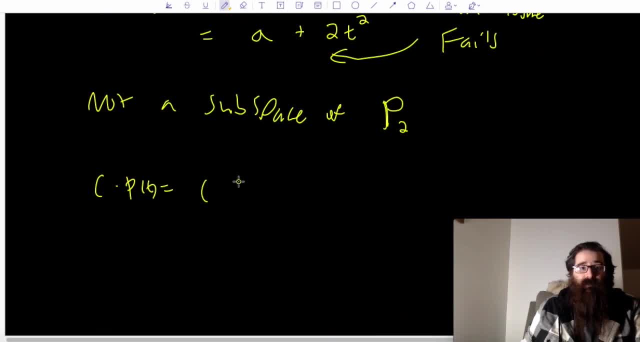 so let's say c times p at t, which would be c times some polynomial of the form a plus t squared. it's really a similar argument. We'll say: well, distributing this in c times a, that's kind of fine. 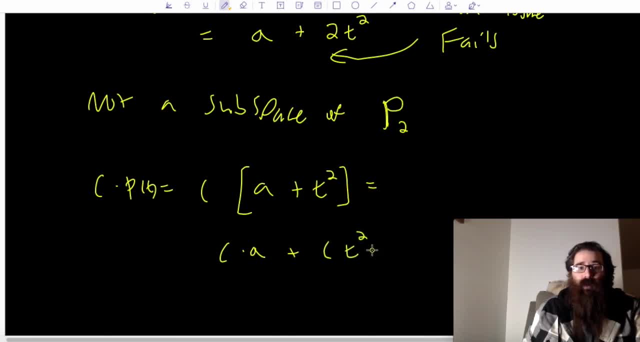 This is still a real number, But then c times t squared. I'm not allowed this. unless c is one, Any other value for c is going to serve as a counterexample. So this doesn't hold true for all scalars c. In fact, there's only one of these that will keep us in that same form. 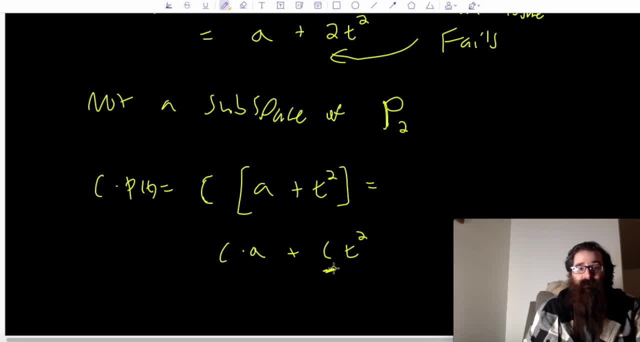 number plus t squared, because now I have this coefficient on t squared again, We'll say, well, so that's going to fail. Another thing to consider is, if I'm looking for that zero element, I'm not going to have it. 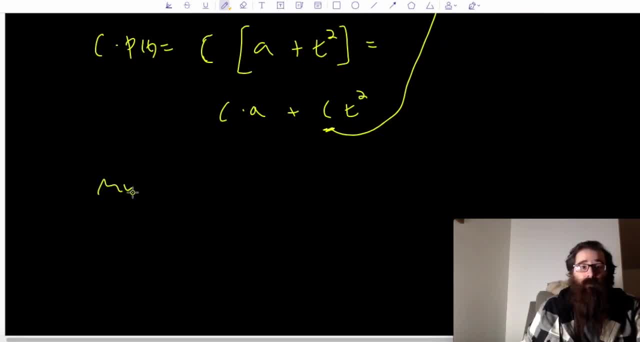 My polynomials must be of the form p at t has to be some real number, a plus my t squared term. Now I have control over the real number, So we'll say: well, this could be any scalar, so why not let it be zero? 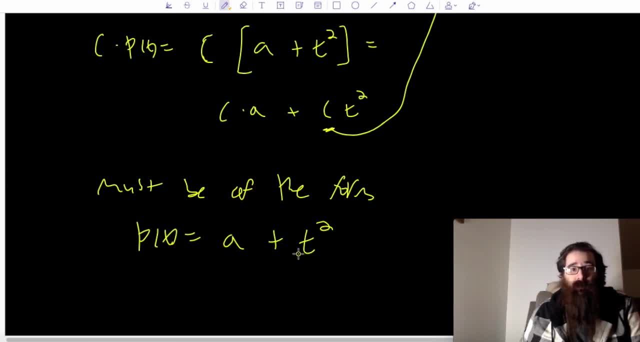 But what I don't have control over is the t squared term. I don't have any coefficient on it. There's no real number in front of this, So there's no way for me to actually zero this out, So I'm not able to achieve the zero element. 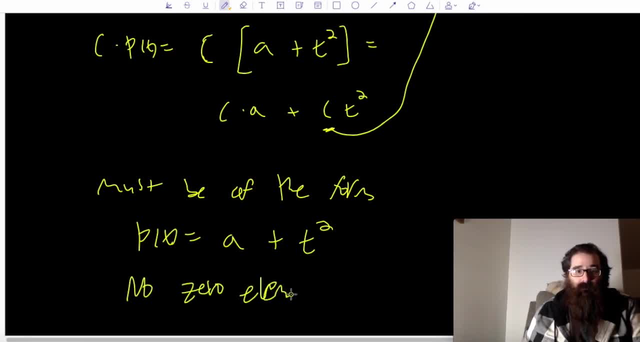 So I'll say no zero element. I would need control over the t squared term, which I'm not given any coefficient there. So the closest I can get is zero plus t squared, but that's not going to give me the zero polynomial. 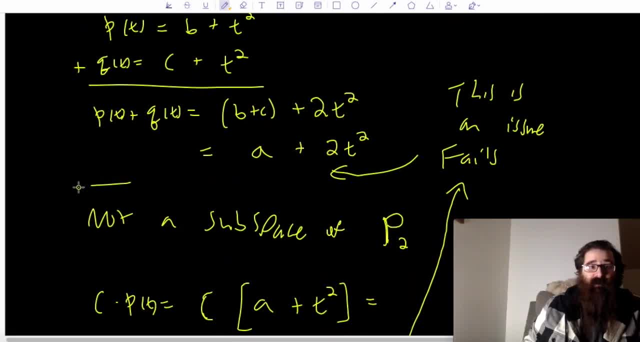 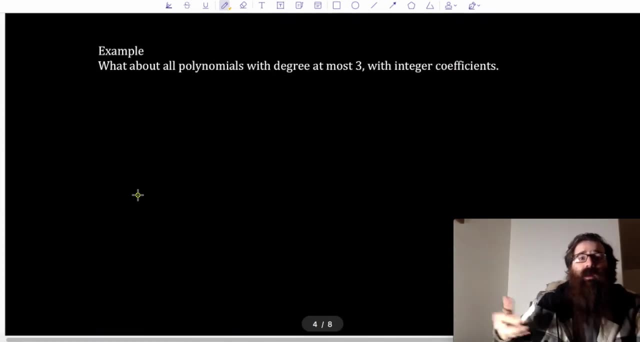 So this is not a subspace of polynomial space p2. And in fact, all three, all three of those pieces that I have to check for a subspace fail. So no good, Well, okay, Well, what about polynomials with degree at most three? 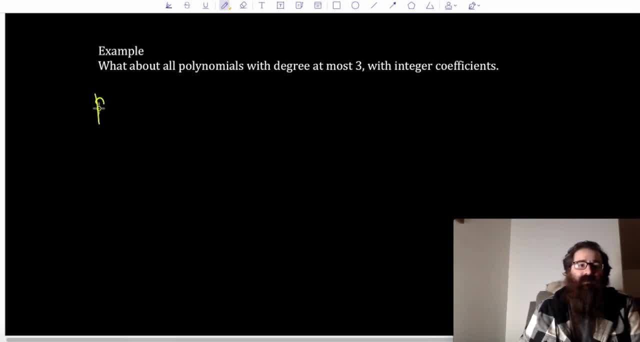 with integer coefficients. So how would this look? Well, we'd say: well, in general, a polynomial would have to be some value. let's say a sub zero plus some constant, a sub 1t plus some constant, a sub 2t, squared. 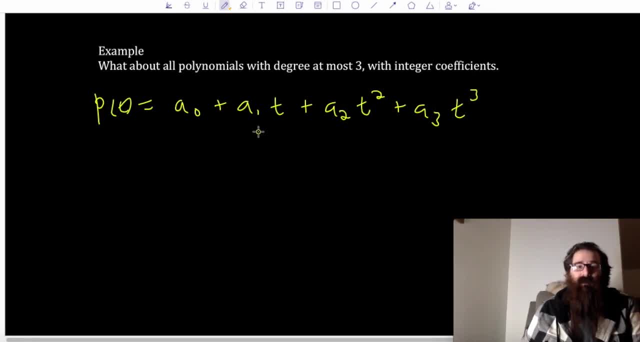 plus some constant, a sub 3t cubed, Where all of these a values must be integers. So we'll write up here: a sub 0, a sub 1, a sub 2, a sub 3 must be integers. 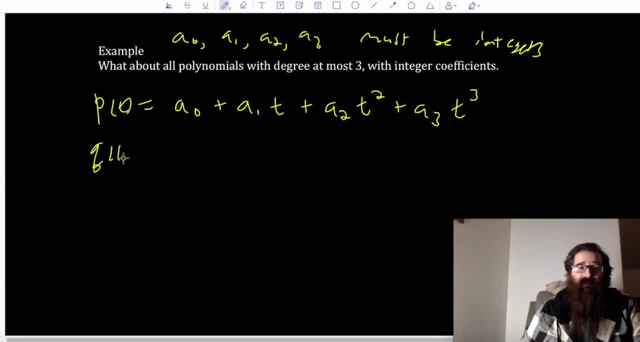 What if I were to take another example of this? So some other polynomial: instead of using a's, let me use b's. but same idea: b sub 0 plus b sub 1t plus b sub 2t squared plus b sub 3t cubed. 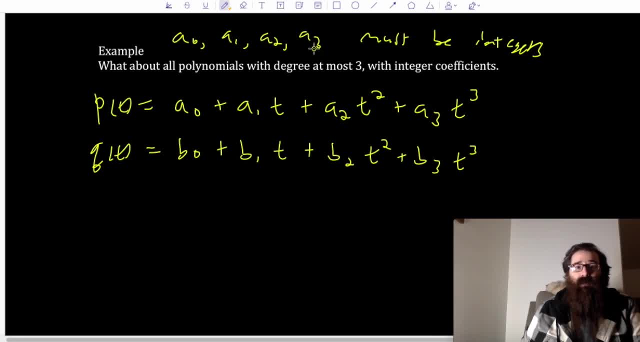 Where b sub 0,, b sub 1, b sub 2, and b sub 3 must be integers. And what if I add these elements together? Well, okay, So if I add my constants together, I'm going to get a sub 0 plus b sub 0.. 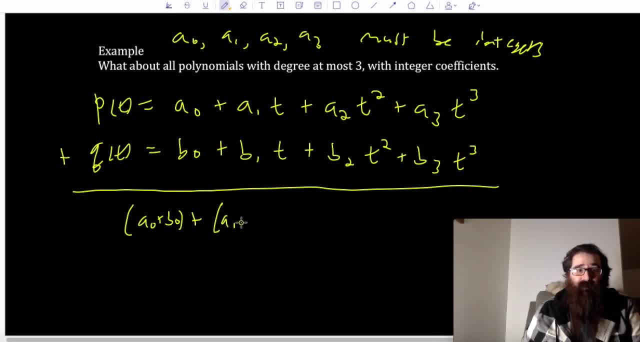 If I add my t terms together and collect, I'm going to have a sub 1 plus b sub 1 times t. If I add my t squared terms together and collect my coefficient, a sub 2 plus b sub 2 times t squared. 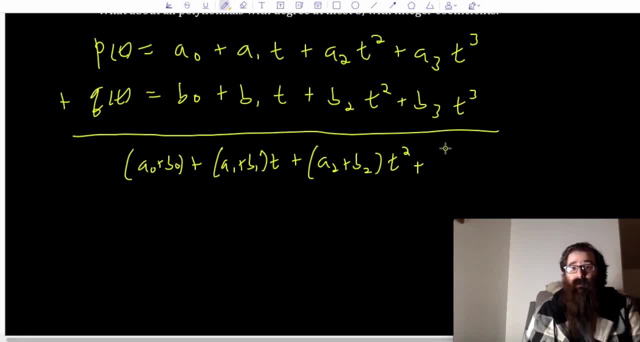 And if I add my t cubed, I'm going to get a sub 2 plus b sub 3 times t squared. I'm going to get a sub 2 plus b sub 3 times t squared And we'll say okay. 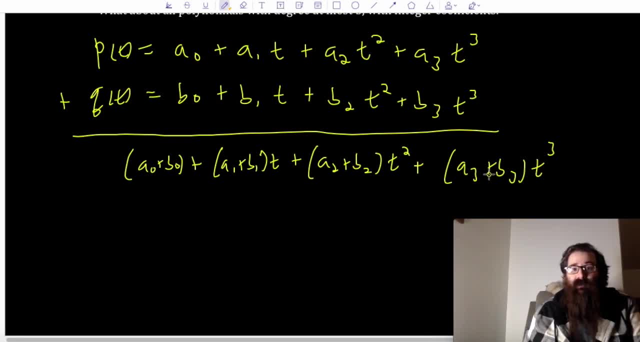 so then, what's going on here? Well, if I add two integers together, that's going to give me another integer. If I take any two integers, add them together, it gives me another integer. I can say: well, this is c sub 0 plus c sub 1t. 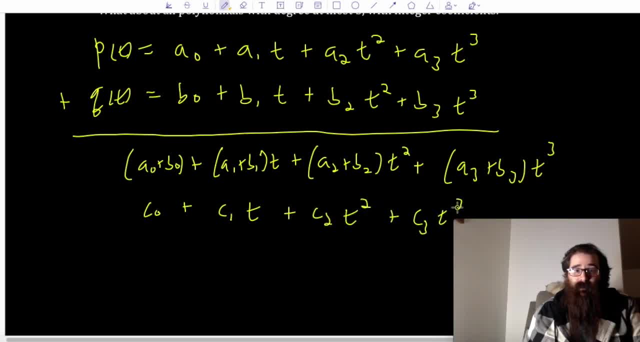 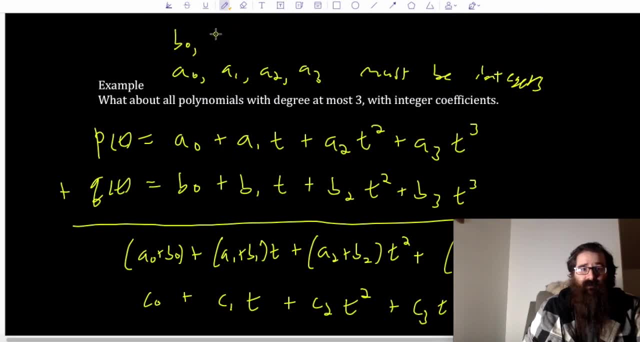 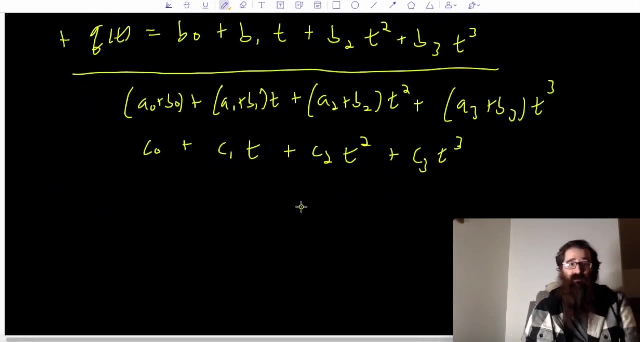 plus c sub 2t squared, plus c sub 3t cubed, And we'll notice that if these a values must be integers- we also said these b values must be integers- then adding these two polynomials together generate another polynomial of degree, at most 3,. 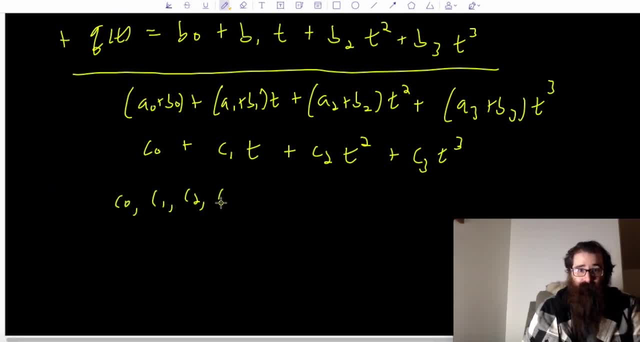 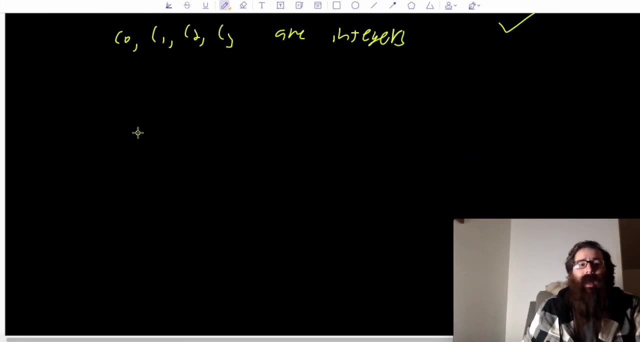 but that the c values are integers. So this works. This works perfectly. What about the 0 element? What about our 0 polynomial? Do we have that? Well, how would that look? So the 0 element would be 0 plus 0t, plus 0t squared plus 0t cubed. 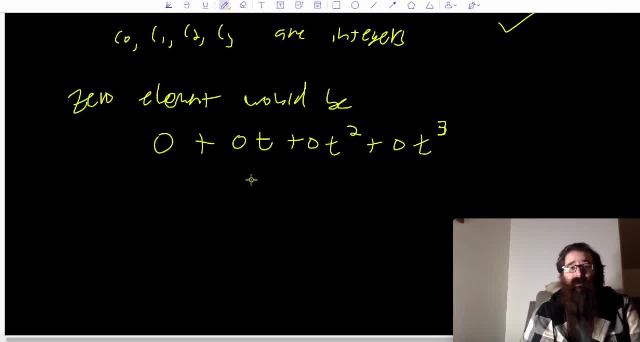 And remember my constants and coefficients have to all be integers. We could say, well, good for us, 0 is an integer, So this works. I do have the 0 element in my polynomial space from the set that I'm describing. 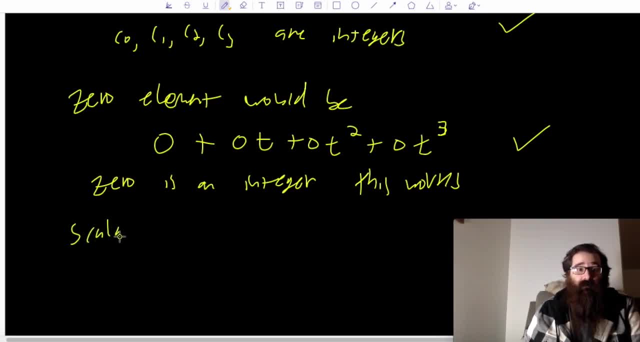 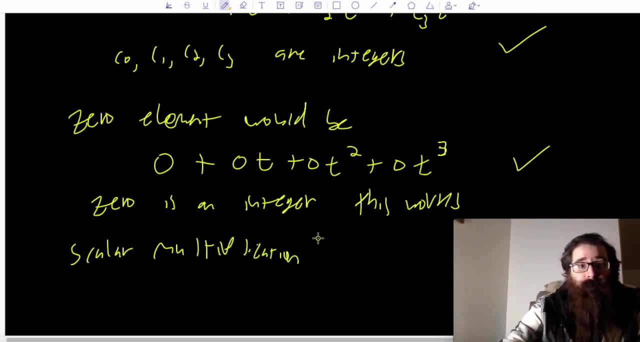 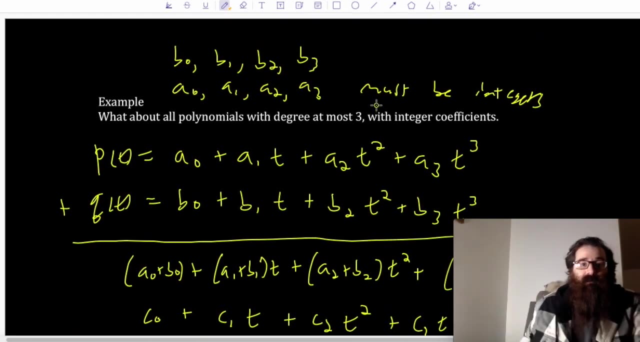 There's one more to check, That's scalar multiplication. Remember, all that we're talking about are polynomials that are degree at most 3, that have integer coefficients. And I want to know: is this going to be a subspace? I didn't write this down earlier. 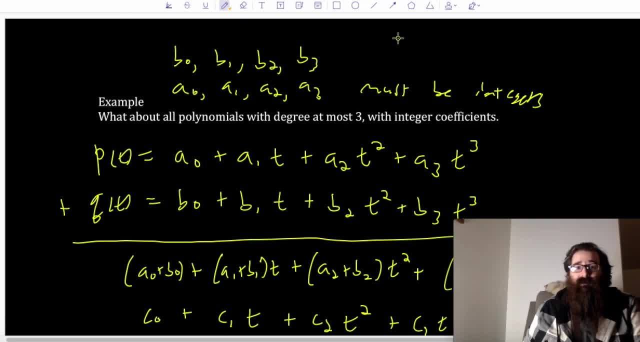 but probably got a good idea. Is this a subspace? I'll write it up here. Is this a subspace? This is a subspace of polynomial space P3, polynomials of degree at most 3? Question mark. I'm trying to find that out. 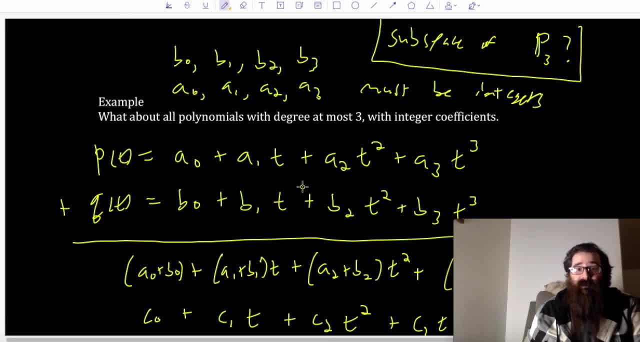 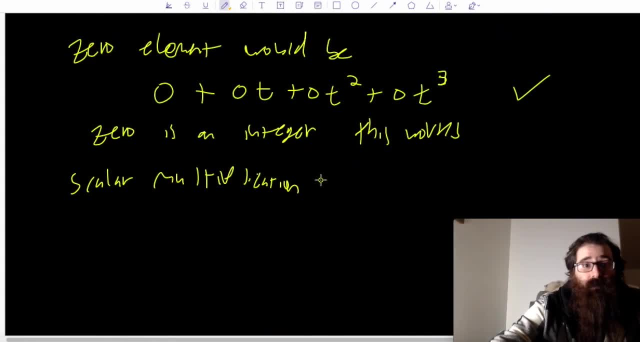 We are closed under addition. If I take two polynomials of this type and add it together, I do get another polynomial that stays in that set. I do have the 0 element. What about scalar multiplication? Am I closed under scalar multiplication? 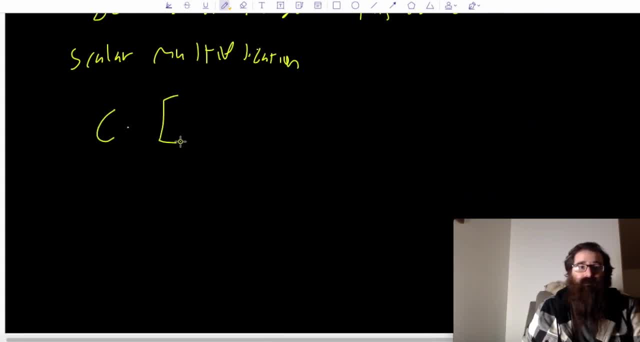 Well, let's see. So if I take a scalar c and multiply it to some polynomial of degree, at most 3, with integer coefficients, a sub 0 plus a sub 1t plus a sub 2t squared plus a sub 3t cubed. 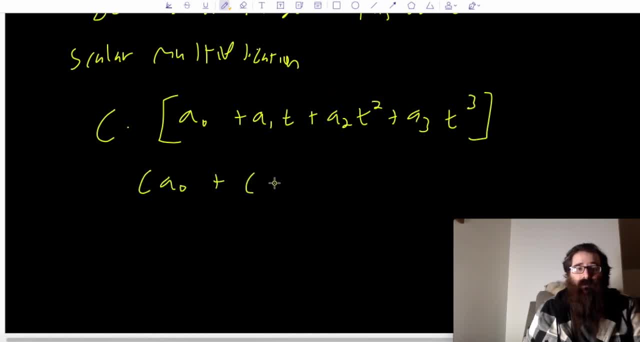 and distribute this through. I'm going to get c times a sub 0,. c times a sub 1 times t. c times a sub 2 times t squared. c times a sub 3 times t cubed. Does this stay where I need it to stay? 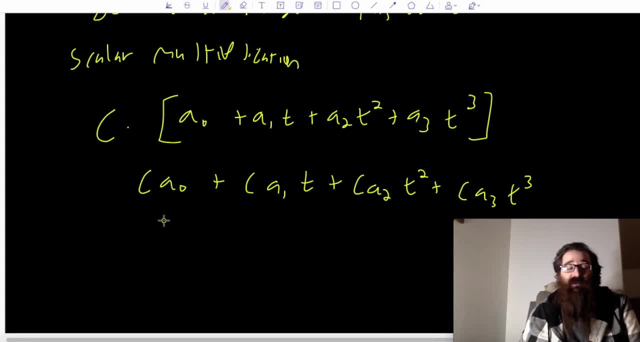 Does it still meet that description? And unfortunately the answer is no. So this is where it actually fails. I was able to get two of the three properties, but this third property isn't going to work out, And you can think of some examples. 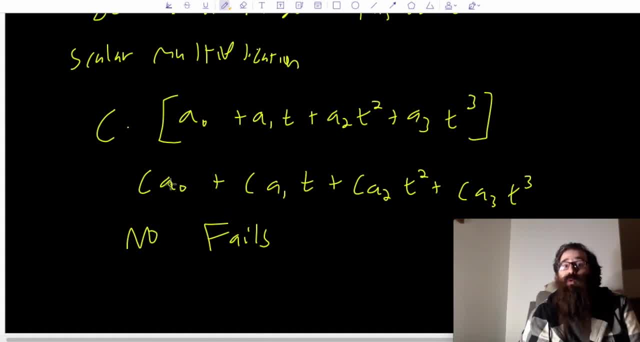 because in fact there are examples that will work for c, but it won't work for any real number. So, for example, what if c is pi? If I multiply by pi, pi times an integer is not an integer, So that won't work. 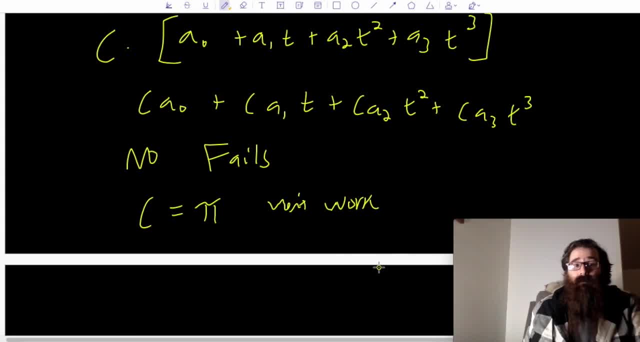 Or my favorite number, e, e won't work either If I take the real number e, e times an integer won't work. That won't keep my integer coefficients. So this we would say: unfortunately this is not a subspace. 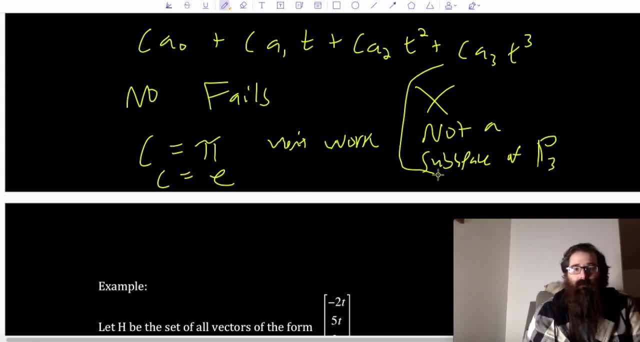 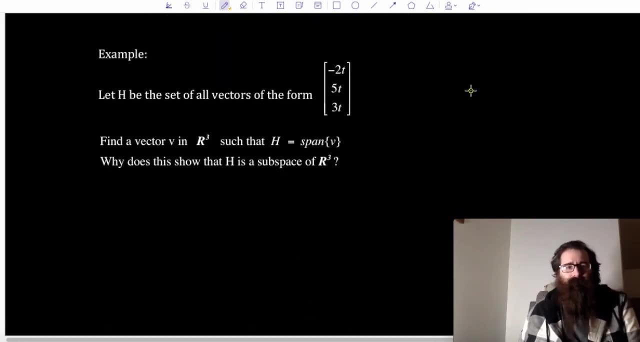 of polynomial space p3. It's a subspace Sad face. Oh, that's happy face. Make it a sad face Depends on how you feel about subspaces. right, Let's take a look at another example, Thinking more about subspaces. 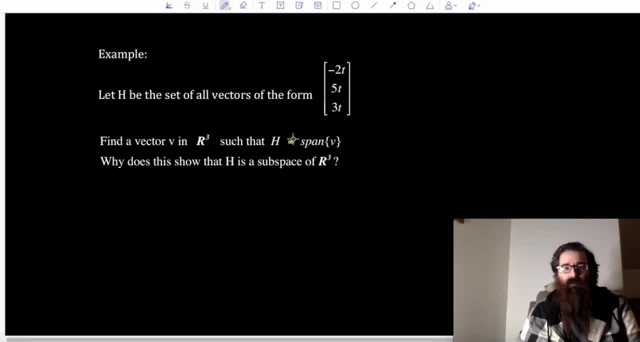 thinking about spanning sets. Spanning sets are going to be very important for the course, And we'll talk a bit more about these in the next section as well. Let h be the set of all vectors of the form, and here I have negative 2t for the first entry. 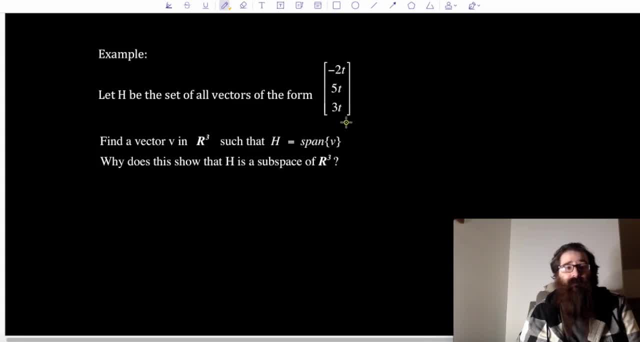 5t for the second entry and 3t for the third entry- And I want to find a vector v in vector space R3, such that h is equal to the span of that vector v. And I want to know: well, why does this show? 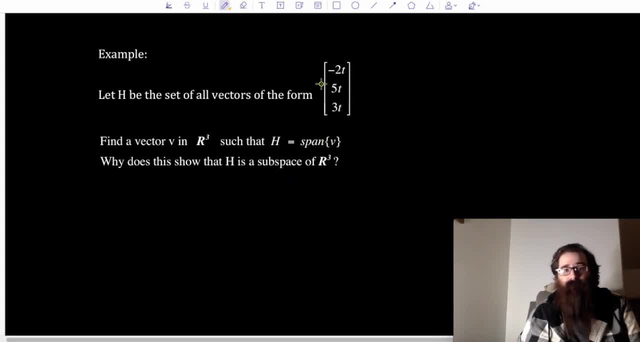 that h is a subspace of R3? Now, this is not going to be a difficult process and we're going to see lots of examples that sort of follow suit with this one. But if I take a vector of this form where the first entry is negative, 2t. 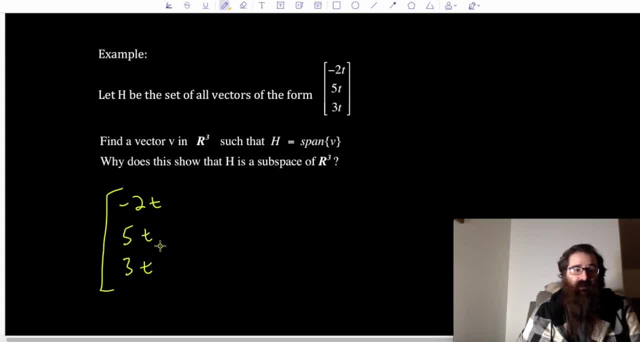 next entry is 5t. the next entry is 3t. I'm probably noticing that I can just factor the t out. We'll do that. Bring the t out, and I'm left with the vector negative: 2,, 5,, 3.. 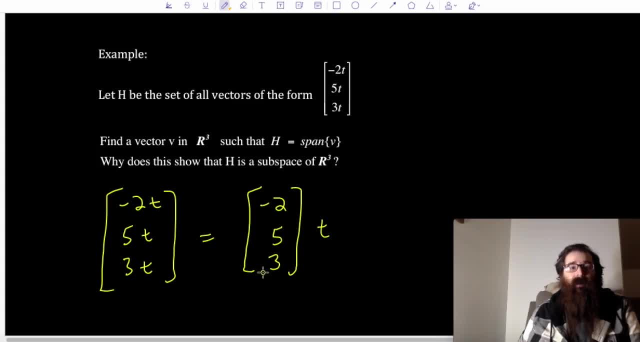 If I multiply the t back in, it brings me back to where I was. But this we're saying that t can be any real number and t is acting as a scalar weight, which means that right now I'm already describing the span of a vector. 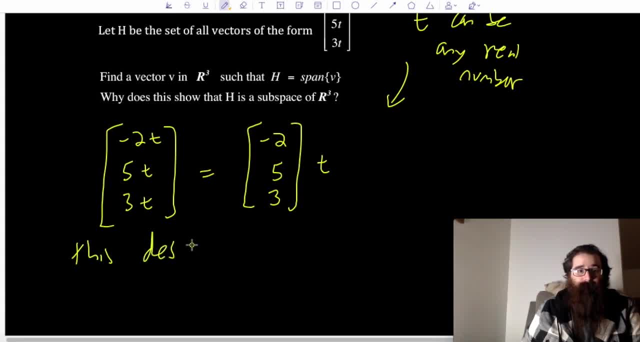 So what are we saying? We're saying: this describes the span of the vector, with entries negative 2,, 5,, 3.. And this, of course, is going to give us a subspace of R3.. So we'll be able to follow up with this and say: 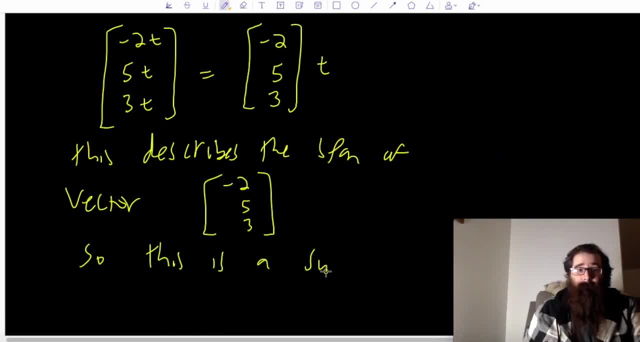 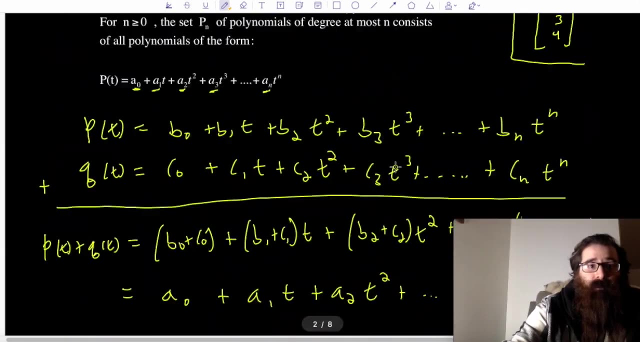 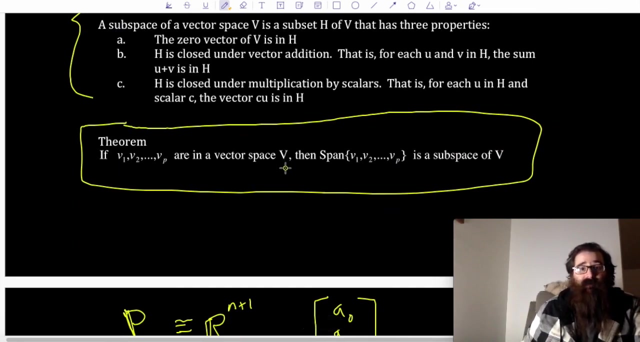 so this is a subspace of R3. Our theorem guarantees this. We have a spanning set that we found. Let's go back and just sort of refresh what that theorem said All the way back. It says: if I have vectors that belong to a vector, space V. 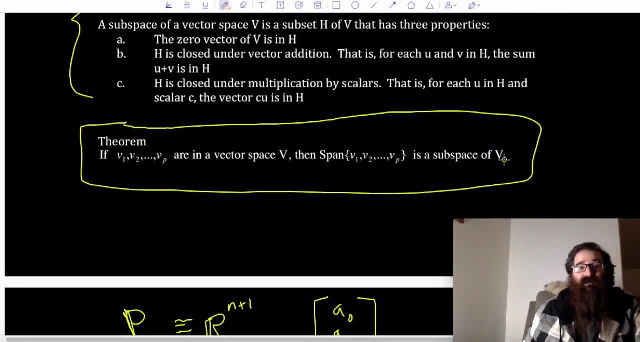 then the span of those vectors is a subspace of that vector space V. We think we talked about span early on in the course. Span is going to be very important for us talking about vector spaces and subspaces, because if I have vectors that live in a vector space, 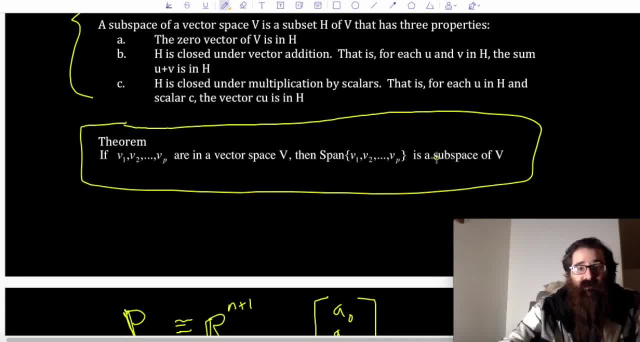 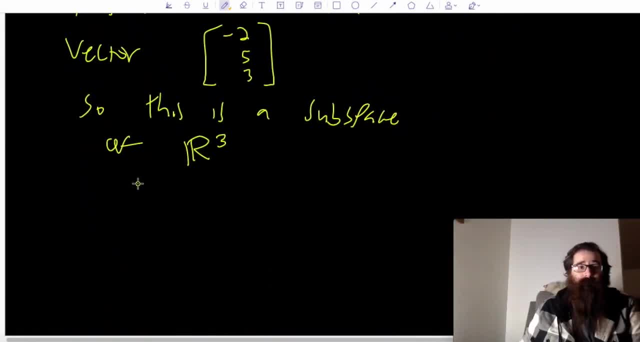 and then I consider the span of those vectors that is going to give us a subspace of that vector space. And what are we saying in our example here? We're saying that this vector, this vector negative 2,, 5,, 3,. 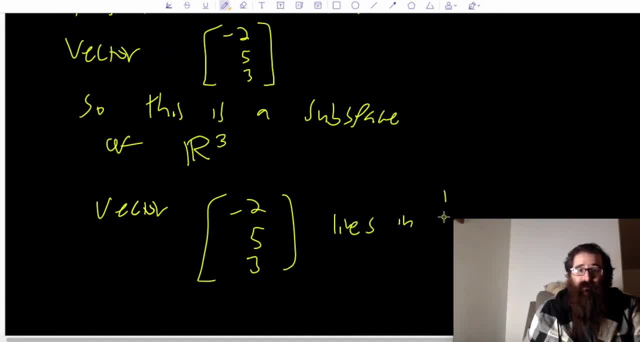 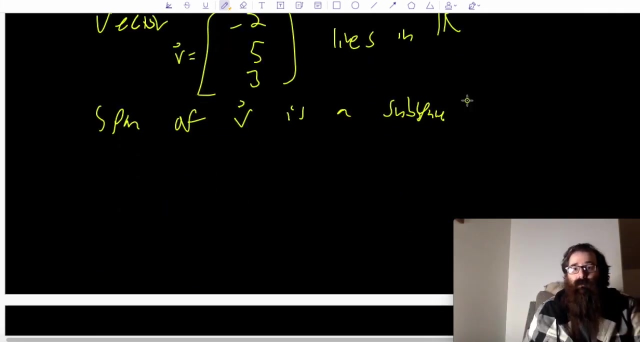 lives in vector space R3. It's got three entries in it. This vector lives in vector space R3.. So then the span we call this vector V, so then the span of this vector V is a subspace of vector space R3.. 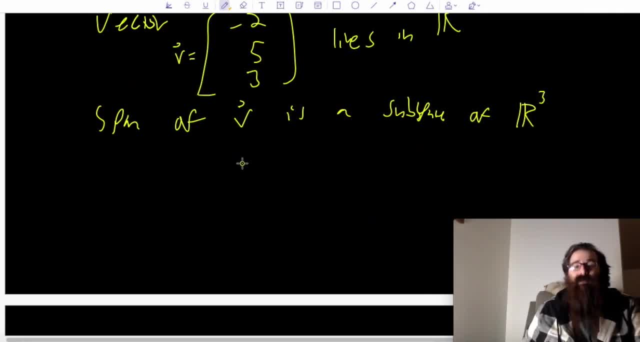 And, if you want to get very specific, this is a one-dimensional subspace of R3. It gives me, it generates a line in R3 through the zero vector and this vector. So this is actually a one-dimensional subspace of R3.. 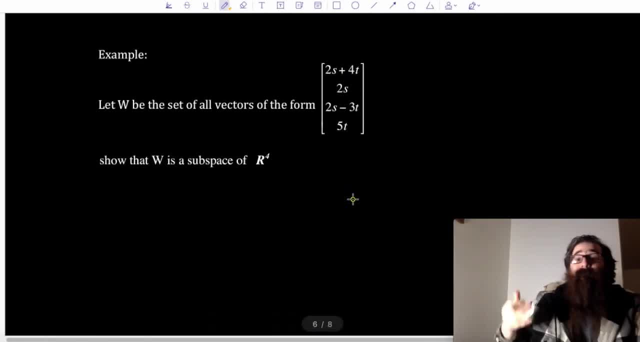 But is in fact a subspace of R3.. It's all about finding that spanning set. So let's see this example, Let W be the set of all vectors of the form. We have. you know, four entries. First entry is 2s plus 4t. 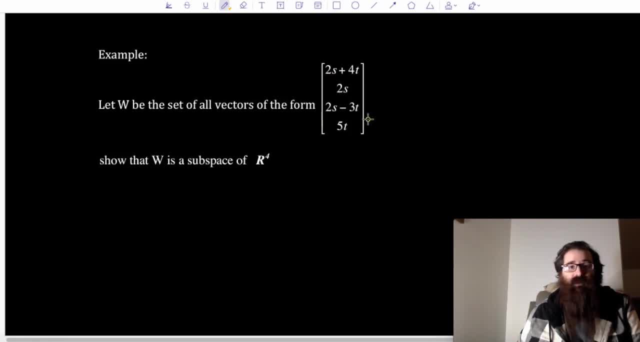 Next entry is 2s. Next entry is 2s minus 3t. Last entry is 5t. Show that W is a subspace of R4.. Let's build a spanning set. So what I can do is I can take this description. 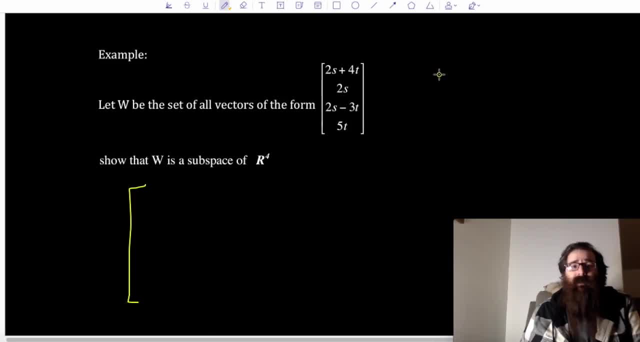 of my vectors. And here we'd make a comment. We'd say: you know, s and t are real numbers. What I want to do is I want to split this into the sum of two vectors: One vector relying on s, one vector relying on t. 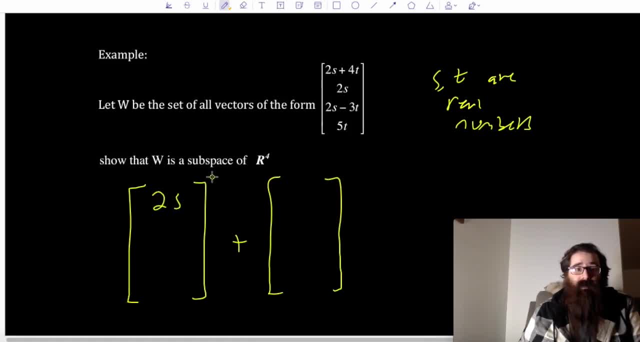 So all of the s's over here, I have 2s, And then another 2s, And then- would you believe it- another 2s, And then, for the fourth entry, no mention of s. So I'm going to write it in any ways as 0 times s. 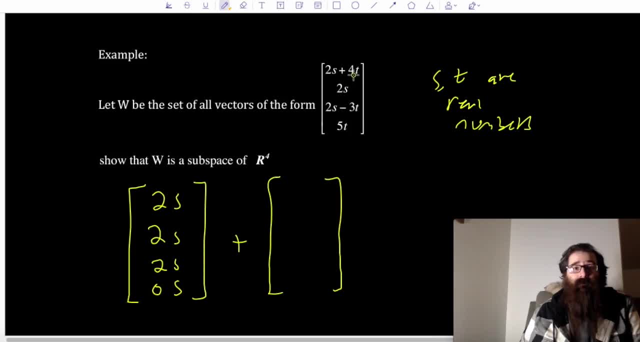 And over here on my next vector, I want all the t terms. That's going to be 4t And then I don't have any t mentioned, So that's going to be 0 times t And then negative 3t. 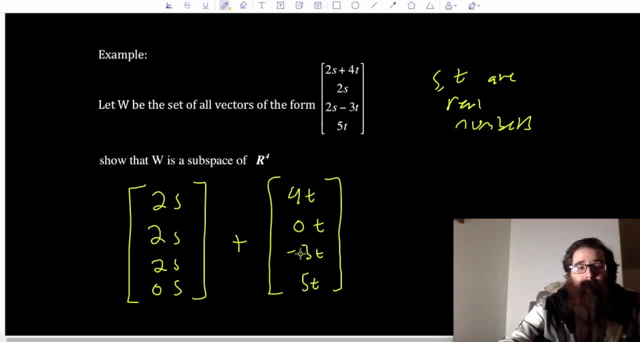 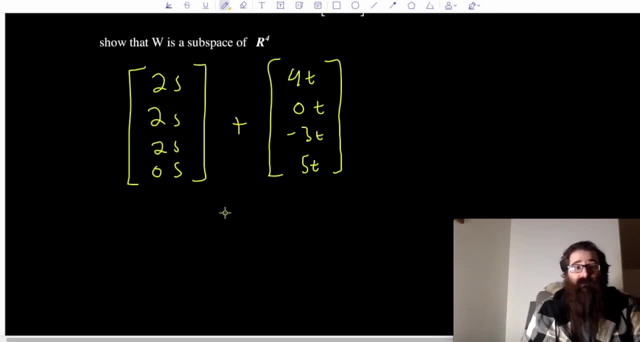 And then lastly, 5t, What I can do, since s and t are just real numbers, think of them sort of like free variables. they're scalar weights, right, Bring s out as a scalar weight from the first vector. 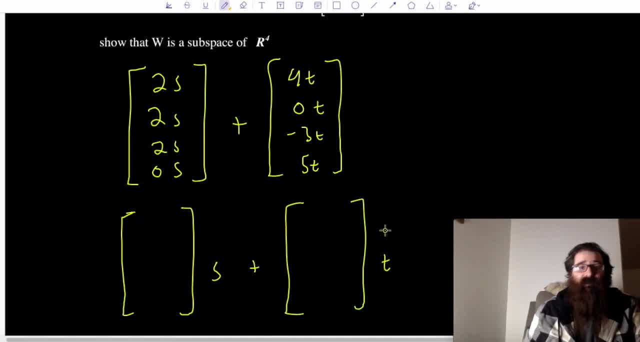 And bring t out as a scalar weight from the second vector And this leaves from the first vector. I'm left with a vector of numerical entries only now: 2,, 2,, 2,, 0. And in the second vector 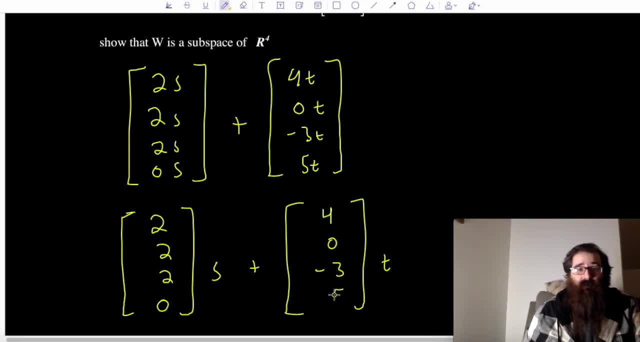 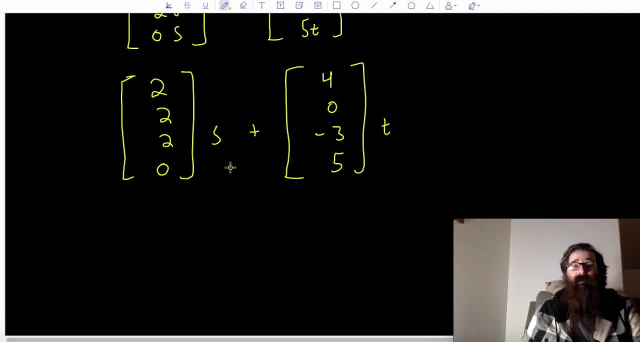 at least behind numerical entries 4, 0, negative 3, 5.. We're saying: well, this describes the span of these two vectors Right. s and t are just real numbers. These are scalar weights now And whatever you'd like for them, 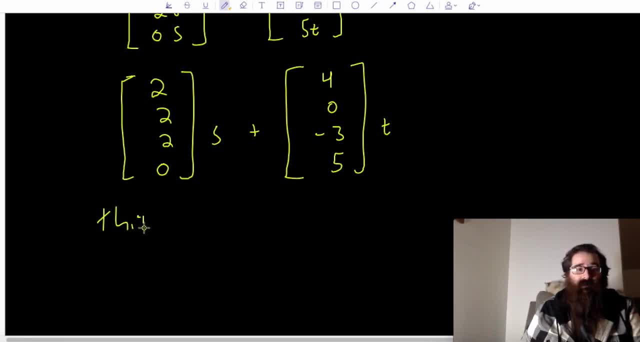 So I'm describing the span of these two vectors. So I'll say this describes the span of vectors. What vectors do we have? We have 2, 2, 2, 0.. And vector 4, 0, negative 3, 5.. 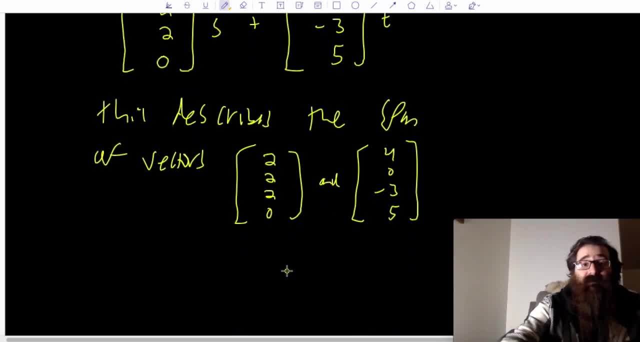 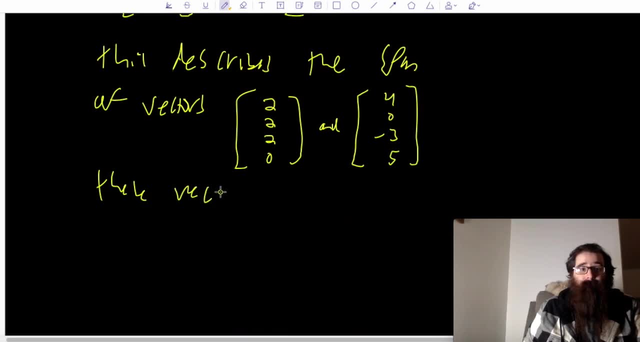 We're describing the span of these two vectors, And these vectors live in R4. They have four entries each: 1, 2, 3, 4, 1, 2, 3, 4.. So let's say these vectors. 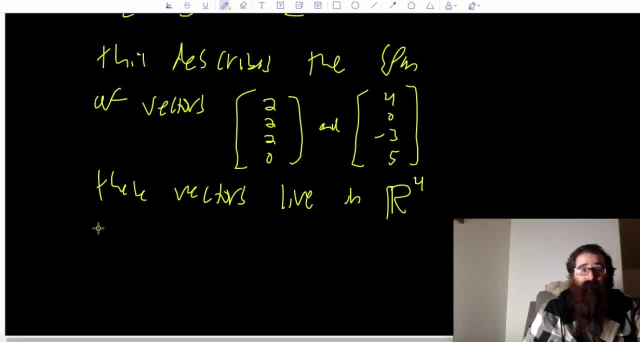 live in vector space R4. So the span gives me a subspace of R4. And, truthfully, this is going to give us a two-dimensional subspace of R4. You have to be careful with just generalizing that type of argument. 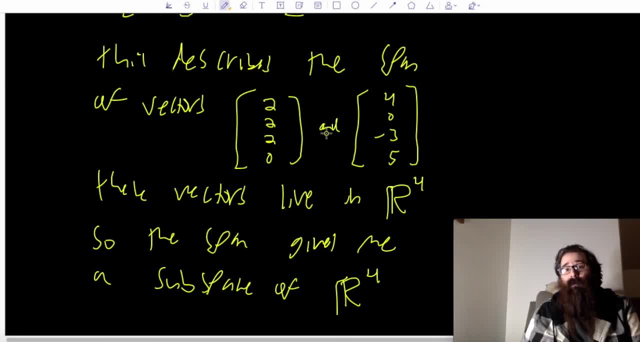 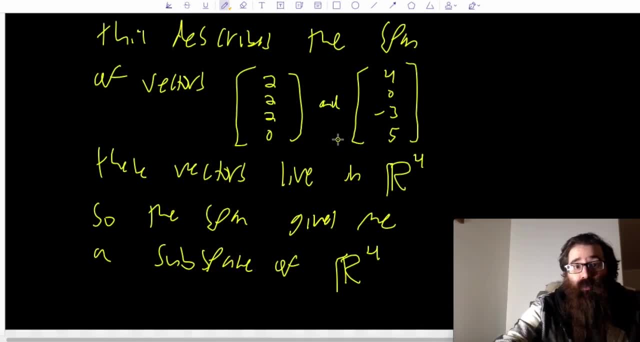 I want to make sure the vectors are linearly independent, But we can probably tell by inspection that well, OK, so these vectors are not multiples of each other. It's more difficult if we have more than just two vectors, But we'll be able to see that these 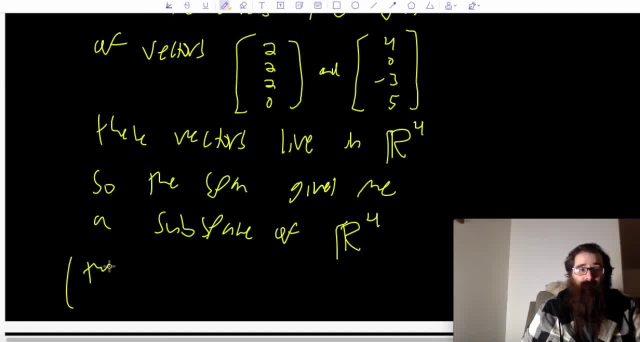 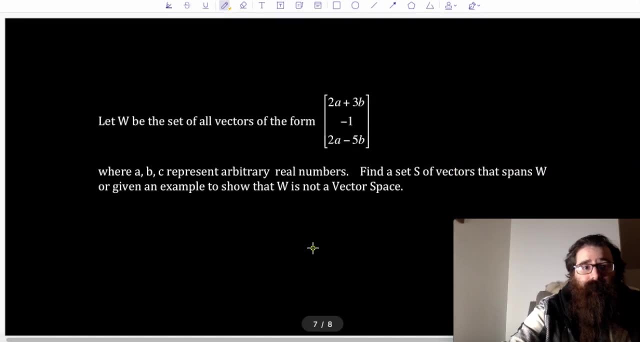 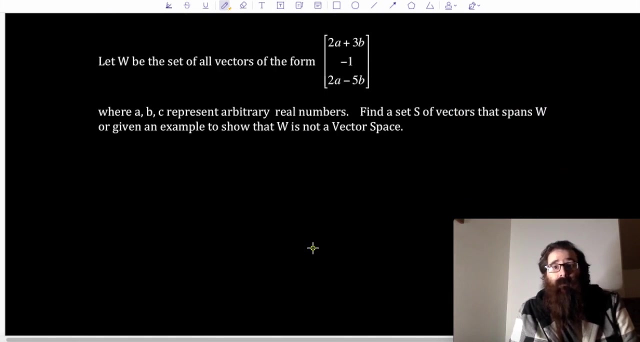 are not dependent vectors. So in fact what we really have here is a two-dimensional subspace of vector space R4. So we do have a subspace of R4. We'll take a look at just a couple more Here. let W be the set of all vectors of the form. 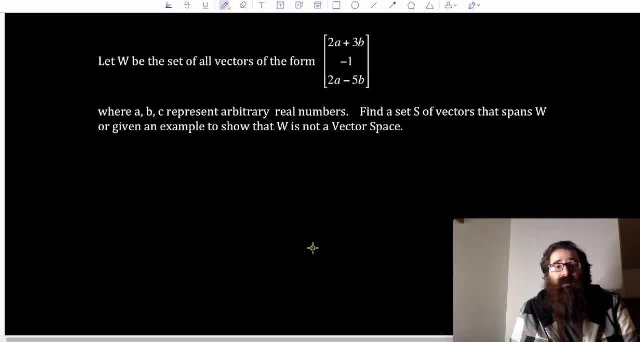 We have a first entry, 2a plus 3b, A second entry, negative 1.. And a third entry, 2a minus 5b, Where a, b and c- And in fact there's no mention of c here- 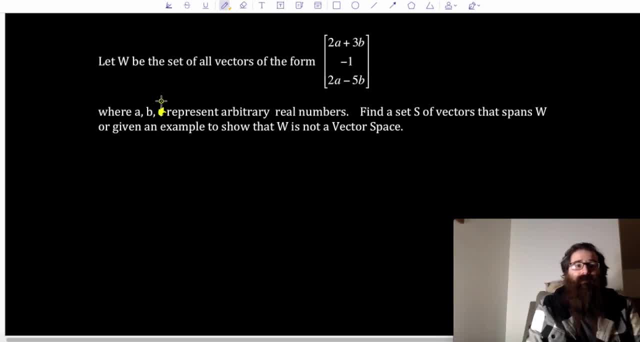 So c for Cory, Where a and b represent arbitrary real numbers. Find a set S of vectors that spans W, Or give an example to show that W is not a vector space. Now you might be looking at this and noticing something a bit different about it right away. 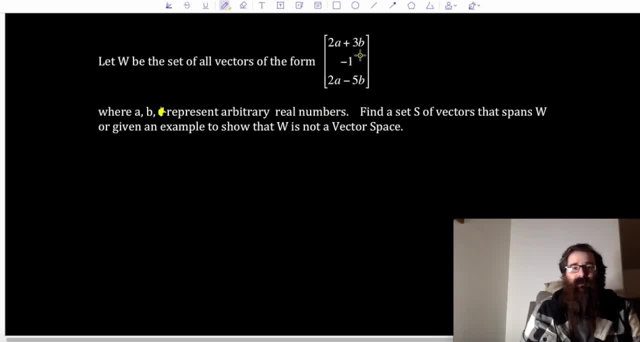 Let's just go ahead and say what it is. That middle entry is going to create such an issue for us. Now, why would it create an issue? Well, right away, we could say: in order for this to be a subspace of a vector space, 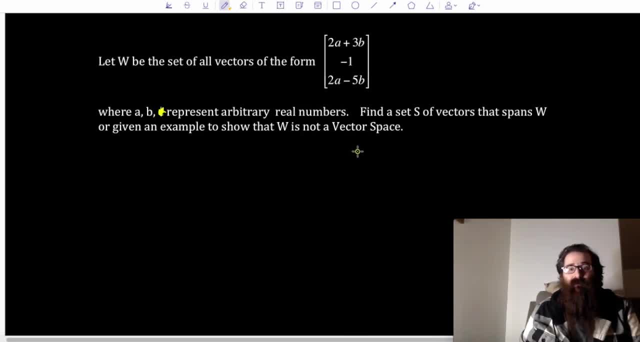 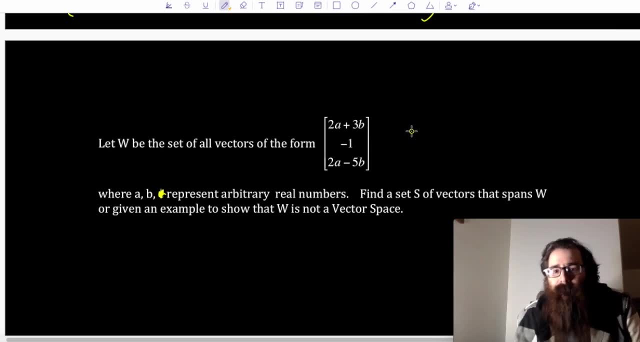 Now let's sort of talk about an idea that we want to sort of continue on with into some future sections. This is going to be a bit of a shortcut for us. Are you ready for a shortcut, for a pro tip from me to you? 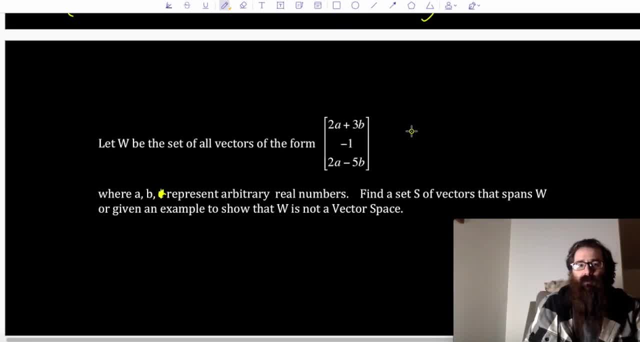 Let me know In the comments section below if you're ready for me to give you this pro tip. And don't tell anyone that I told you Because I don't want to get in trouble. I want to stay on good terms with everybody. 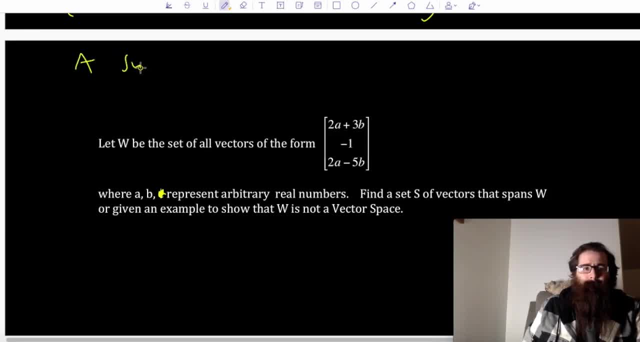 So we'll say this: A subspace of a known vector space is itself a vector space. If you can show that something is a subspace of a known vector space, then that's going to serve as its own vector space as well. So in fact, you could go and you could show. 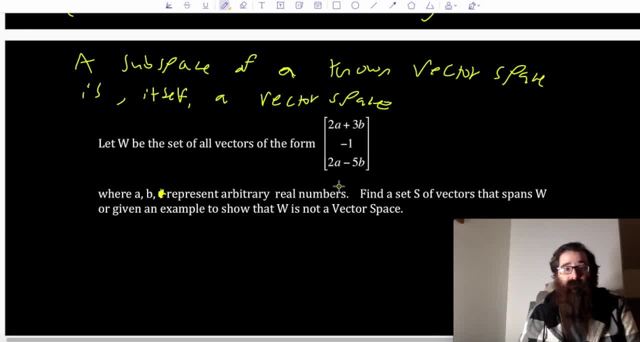 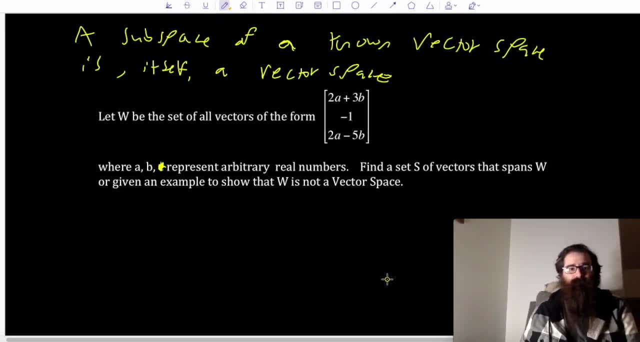 that the remaining axioms do hold true, which is going to be very fantastic. I stay inside of that space. So subspace of a known vector space is also a vector space. So let's go ahead and take a look at what it is we have to say here. 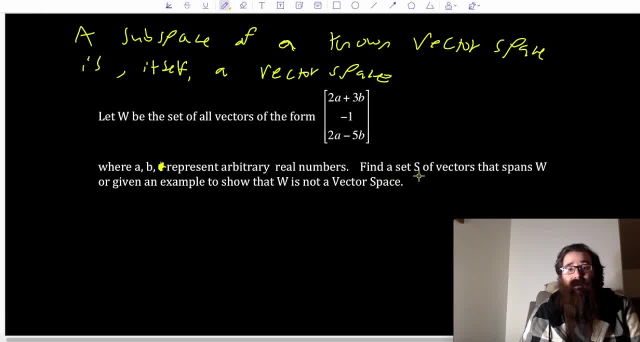 I want to show either that I can find a spanning set or show that W is not a vector space. Okay, Well, right away, there's some consideration to make. I think about that second entry. I think about maybe the zero vector. first, 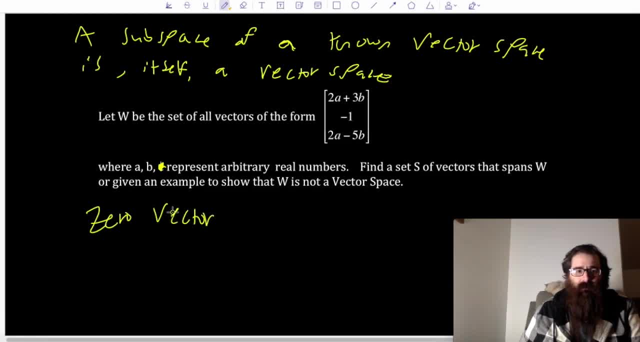 The zero vector is a good place to start here. How would the zero vector look? Well, these are vectors that live in R3.. I have three entries. The zero vector of R3 would have to be 0, 0, 0.. 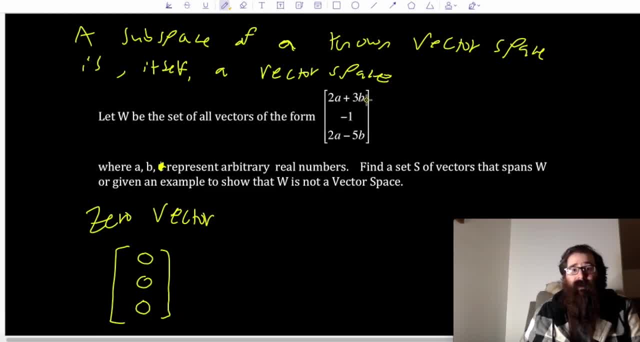 Will that work? The first entry is fine, right, A and B are real numbers, and if A and B are both 0 or if there's some balancing going on between them, I can get 0 out of that. What about for the third entry? 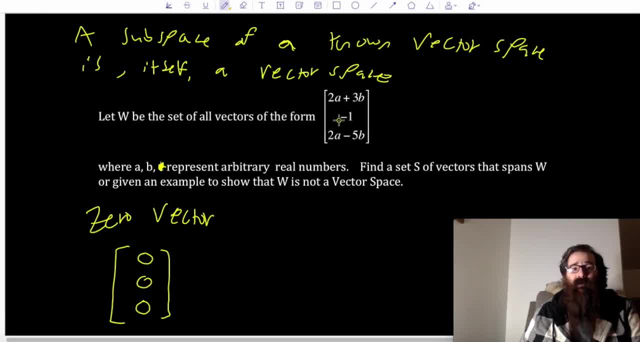 Sure, that could be a possibility, but not at all for the second entry. The second entry must be a negative 1.. So second entry must be negative 1.. This is an issue. Sad face, I don't have the zero vector. 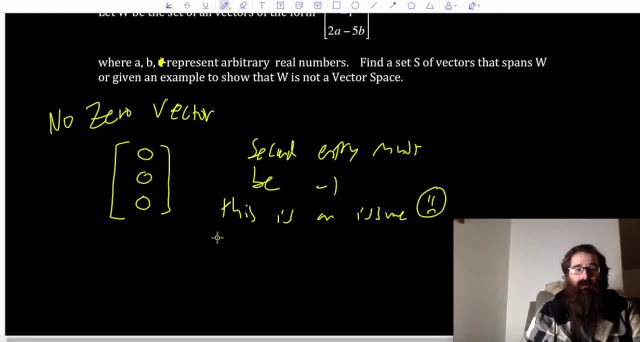 so I'll say that there's no zero vector in our set. That's not the only issue, right? In fact, if I want to show that I'm closed under addition, I'm not. That's not the case If I go ahead and take two vectors of this form. 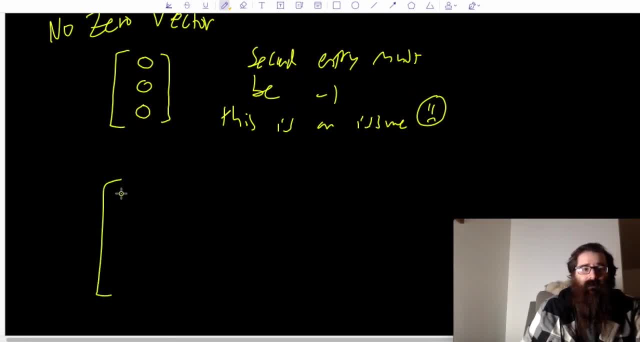 let's say I have a first vector that's 2A plus 3B. We do 2A0 plus 3B0 and then negative 1.. And then what was it? It was 2A minus 5B. 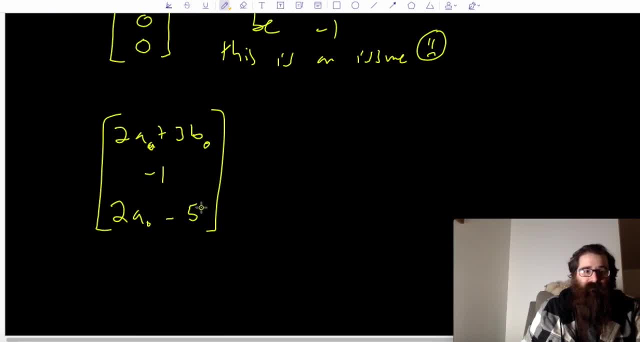 so we'll do 2A0 minus 5B0.. And then I take another vector of this form. so just different scalars. First let me do 2A1 plus 3B1, and then negative 1, for the second entry has to be: 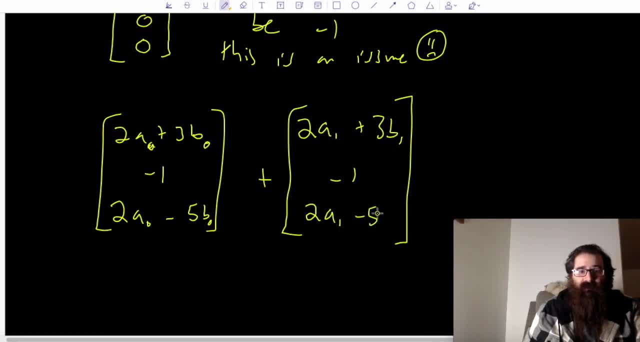 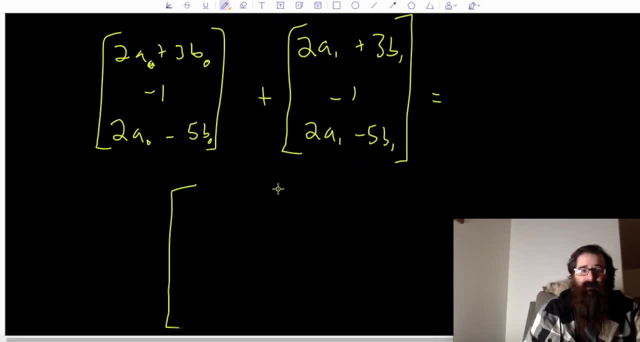 And then the third entry would be 2A1 minus 5B1.. If I add these together, you're probably going to see what's going to happen with this. I can collect. So if I think about adding together, I'm going to have 2 times some real number. 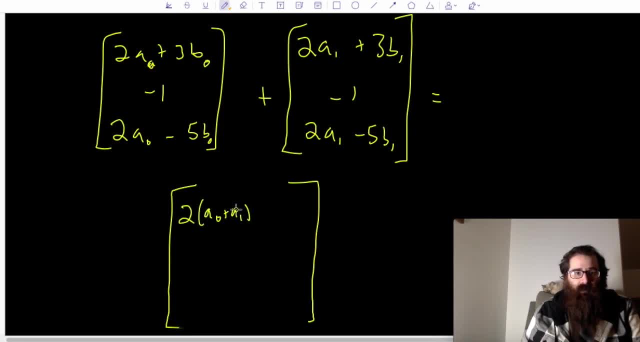 but that collected real number is A0 plus A1, and then plus 3 times the real number, B0 plus B1.. The second entry- this is the issue I'm going to have- negative 1 plus negative 1 gives me negative 2.. 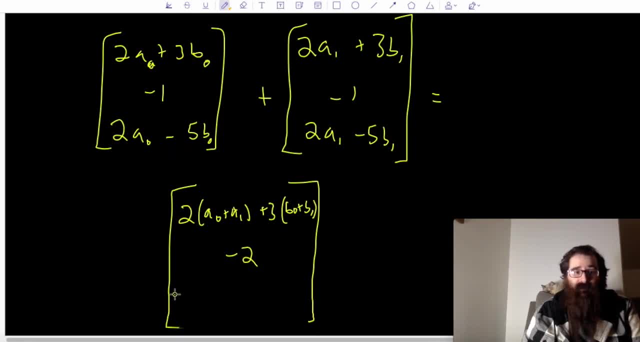 And then for the third entry, it's going to be 2 times some real number. That's going to be 2 times A0 plus A1, and then minus 5 times a real number. That real number is going to be B0 plus B1.. 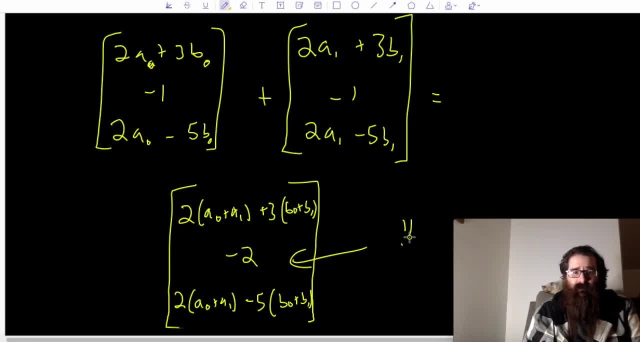 So it's that middle entry that gets messed up. So we'll say, well, what is this? I can't do that. I'm supposed to have this middle entry just be a negative 1, not supposed to be a negative 2.. 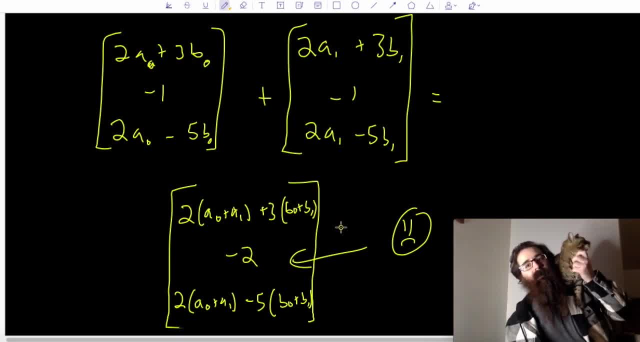 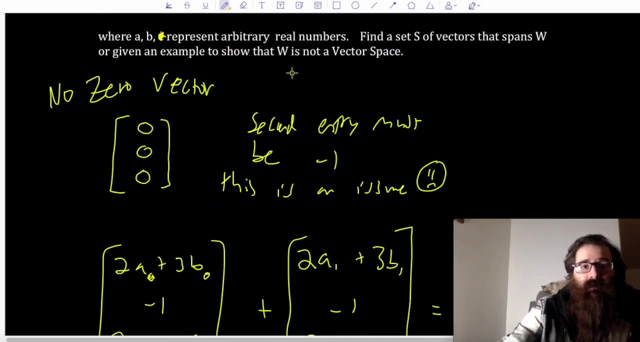 What is the meaning of this? Can't do it Bad, Not good, No, no good. So we'll say, well, this fails as well. So, in fact, what we have here with our set say this set W is not a vector space. 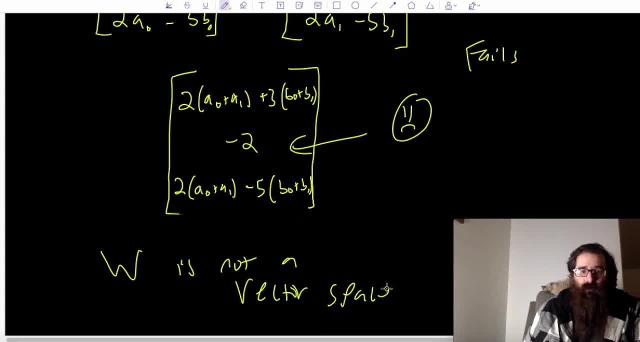 I don't have the zero element. I'm not closed under addition. Issues with scalar multiplication as well. right, If I multiply a scalar times negative 1, I can't guarantee that it's still going to be a negative 1, right. 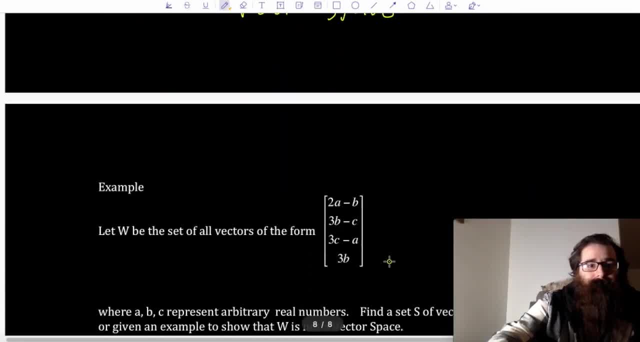 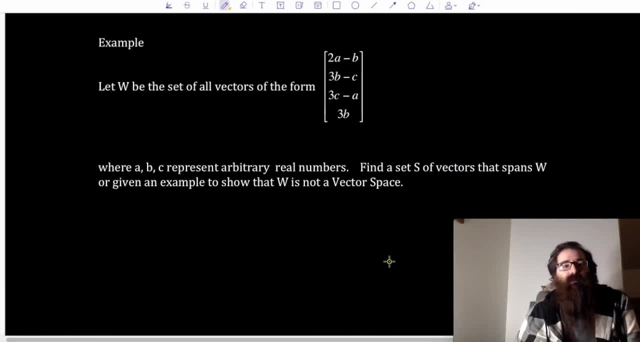 In fact most likely not. Let's take a look at one more example and then we'll head on out for the day. Let W be the set of all vectors of the form We have. first entry: 2A minus B. second entry: 3B minus C. 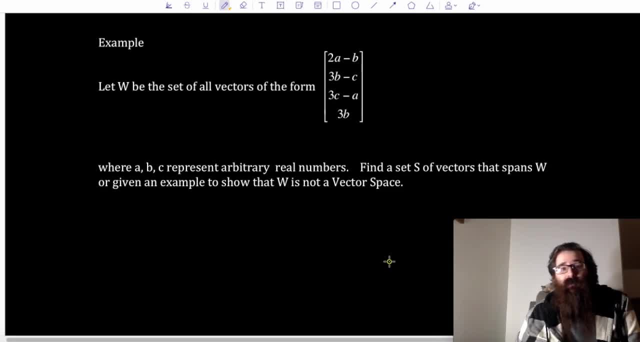 third entry, 3C minus A, and a. fourth entry, 3B, where A, B and C represent arbitrary real numbers, And I'd like to find a set S of vectors that spans W or give an example to show that W is not a vector space. 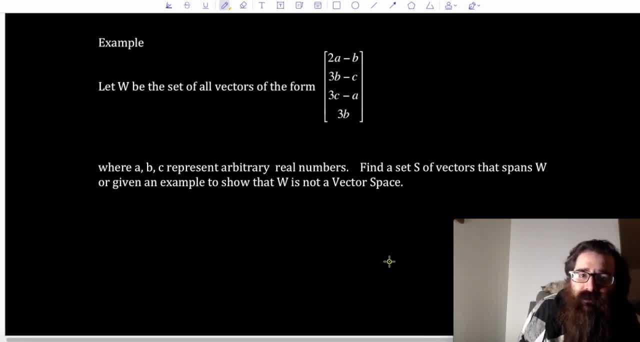 We'll say: okay, well, let's see what's going on here. This actually looks like we could have some success with it. It doesn't look like I'm right away noticing anything suspicious about it. So what could I do? Well, I could try to split this up into three vectors. 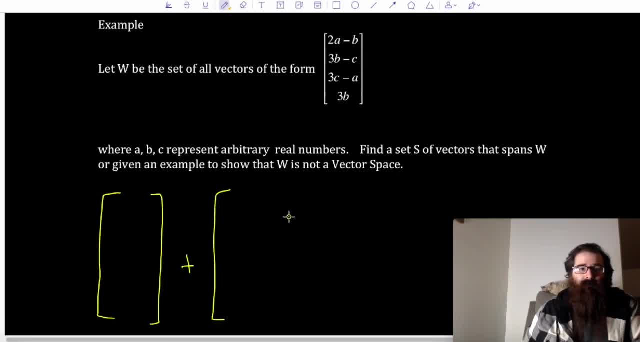 one vector relying on A, plus another vector relying on B, plus another vector relying on C, And I can try to build a spanning set Now relying on A, and I got to be careful because things kind of jump around a bit. but I have 2A for the first entry. 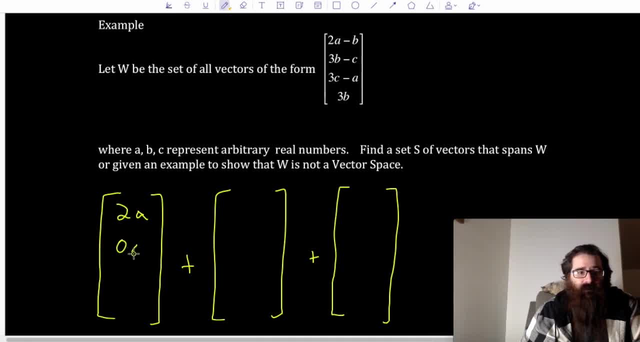 Looks good. Nothing in the second entry, so 0A. Third entry: I have minus A- Say minus 1 times A- And then nothing for the fourth entry, so 0A. What about B? So I have minus B or that's negative 1B. 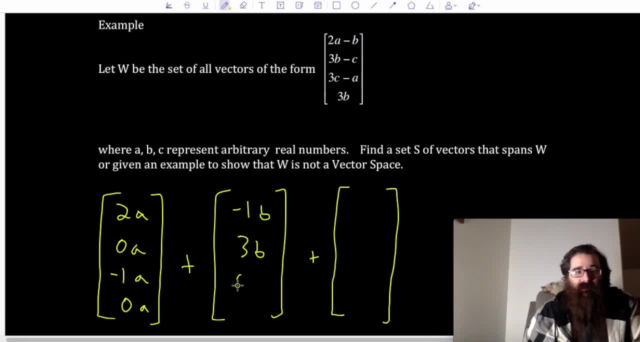 3B. Third entry is missing. it so 0B, And then 3B for the last entry. And what about C? First entry is missing. any mention of C. so that's 0C. Then I have minus C or that's negative 1C. 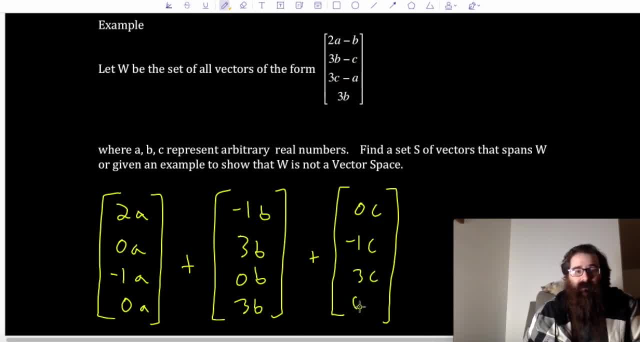 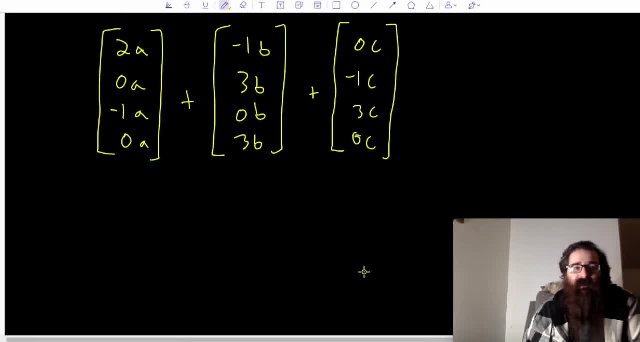 And I have 3C And then I'm missing C in the last entry. so that's got to be 0C. But then A, B and C are just arbitrary real numbers. Think of them now as scalar weights and bring them out. 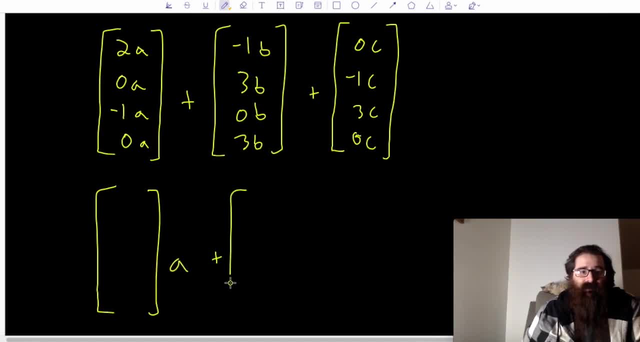 So some vector times A, plus some vector times B, plus some vector times C, And this is going to leave behind vectors with numerical entries only. So this first vector, you guessed it right, It's going to be 2, 0, negative 1, 0.. 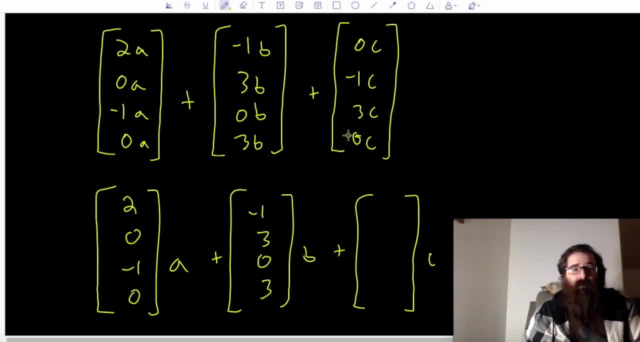 Second vector is going to be negative: 1, 3, 0, 3.. Third vector is going to be 0, negative 1, 3, 0.. But this is now showing that I have the span of these three vectors. 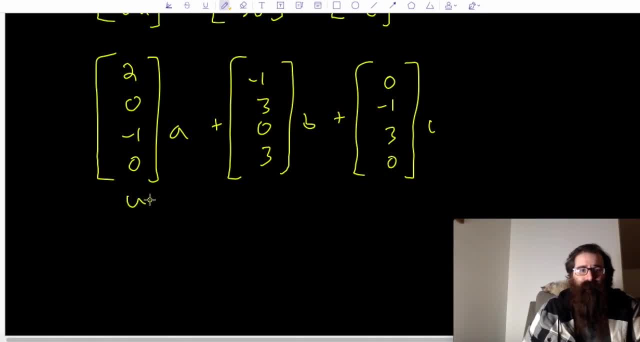 If I want to sort of nickname these vectors U, V and W, what I have is I have the span of U, V and W where these vectors live in R4. So this is going to give me a subspace of R4.. 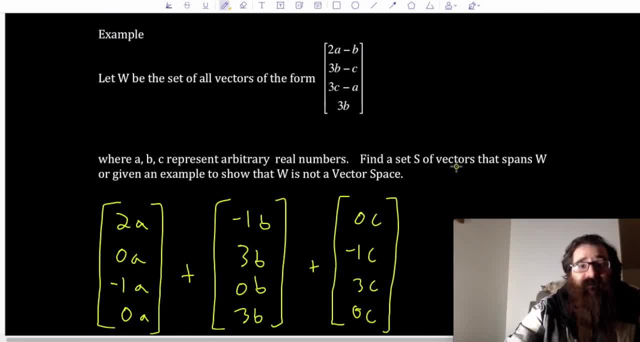 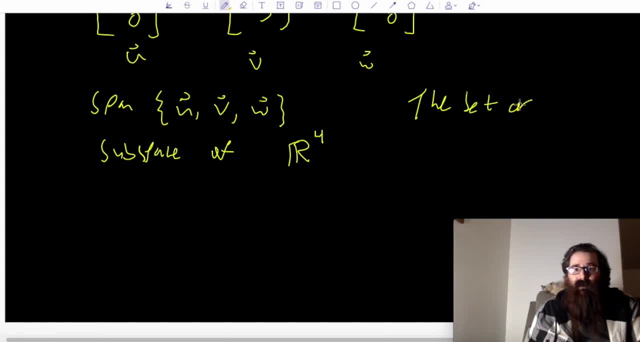 I have a subspace of R4. So the question said: find a set of vectors that spans W. So I can do that. now I can say the set of vectors that spans W is going to have a set. The set's going to have three vectors in it. 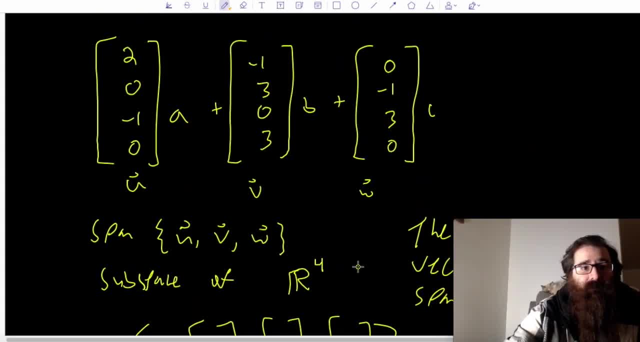 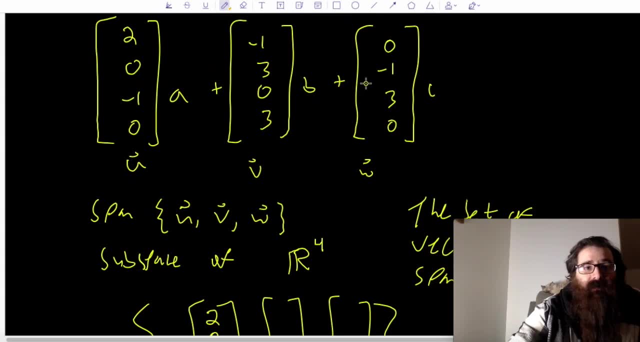 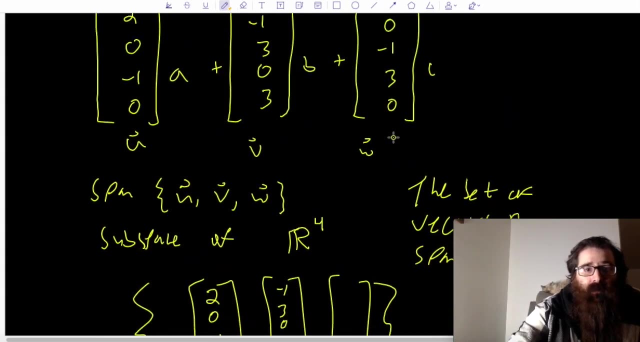 That first vector is going to be 2, 0, negative, 1, 0.. Second vector: negative: 1, 3, 0, 3.. And the third vector is going to be 0, negative 1, 3, 0.. 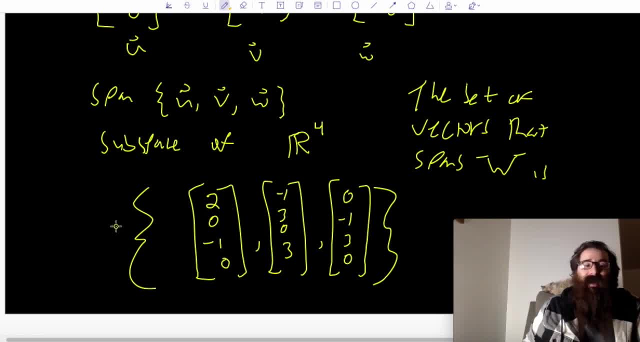 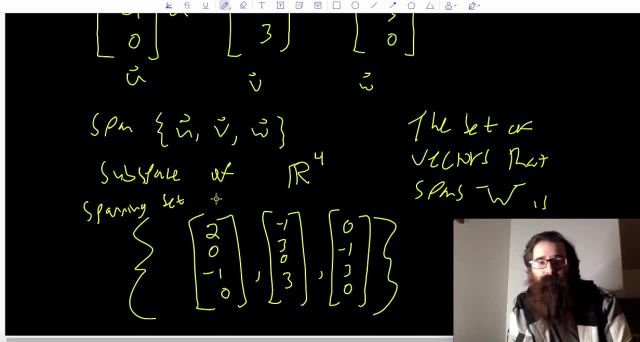 And this is going to be my spanning set. Let's use that term right now Because we're going to be using it later on in the course as well. I have this spanning set. Hey, let me know what you think about all of this vector space and subspace stuff.